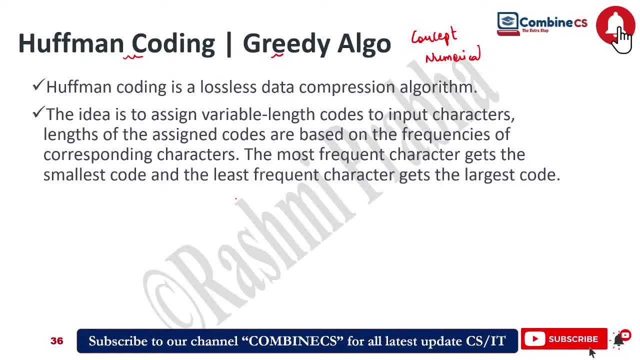 So what is halfman coding? I will explain it to you in a simple way. So this is a tree structure. In this way, we will make a tree In this tree. you have to understand that there is a property of heap. What is heap? 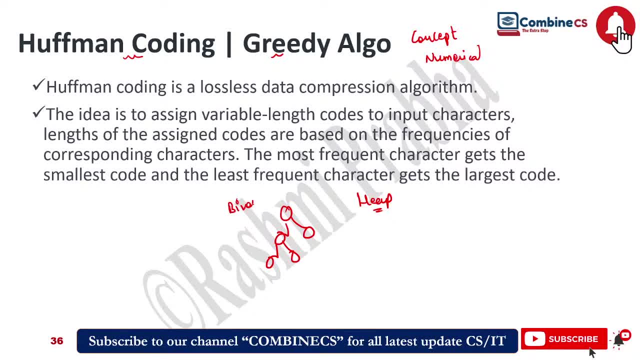 So in heap, we have to understand that this is one of the binary tree. In binary tree, as we know that heap will be of two types: either it will be max heap or minimum heap. This is the meaning of max heap, which is your root node. 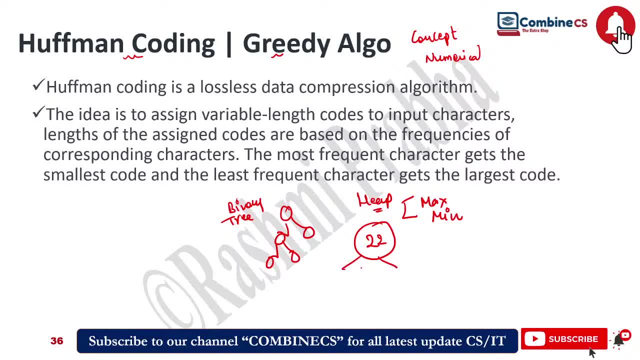 Which is always bigger than your child node, Which is always bigger than your child node. That is, if I make it 15, then you can make it 20 here It depends on what value you are taking. If we talk about minimum heap, it is the reciprocal of max heap. 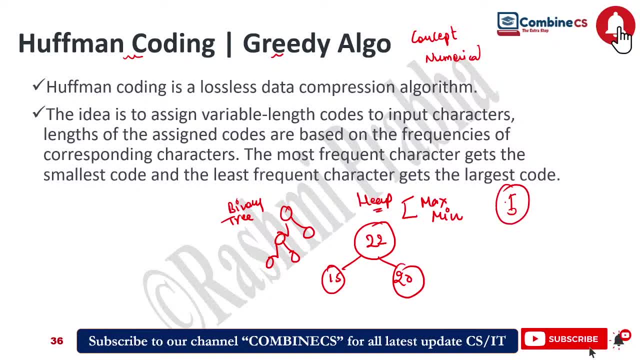 That is, if I write 5 here as a root node, then here we write 1 and here- sorry, if I am writing 1, then here will be 2 and there will be 3.. This is minimum heap. So what will we do in halfman coding? 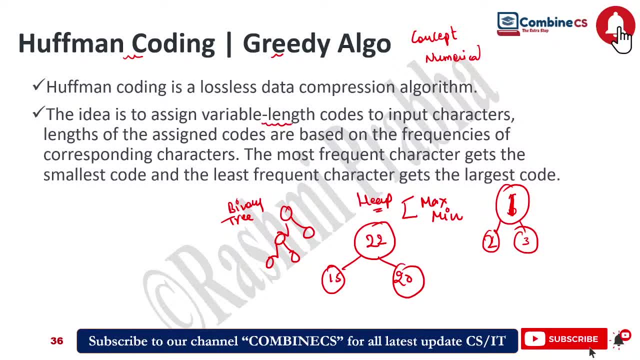 There are certain values. On the basis of those values, what we find out? We find out its code That is used for compression and decompression algorithms. So let us first understand it from a theoretical point of view. We will first look at a practical question. 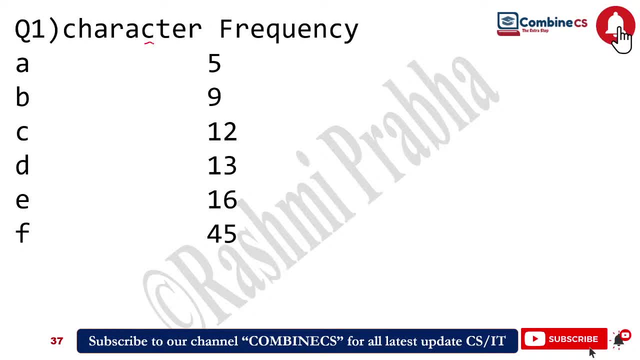 So how will your question come in UDCnet? They will give you some characters And they will give you the frequency And after frequency they will ask you its total value. Otherwise, they will ask you a sequence That is known as prefix node. 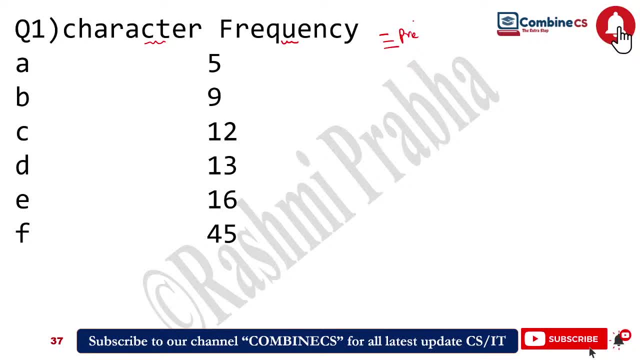 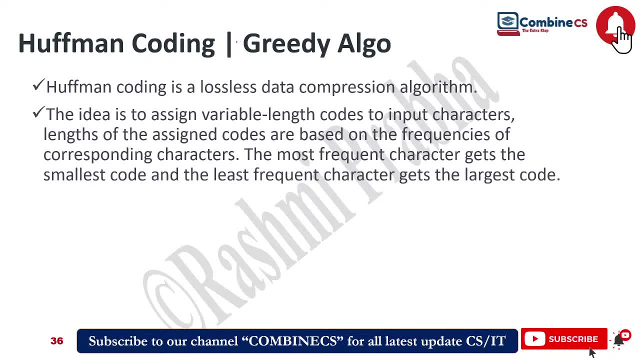 Prenix node. Here we understand the approach of solving this question. But before that, Now Halfman coding is what It is: a lossless data compression algorithm. So this was asked in UDCnet previous year question That you were given options there. 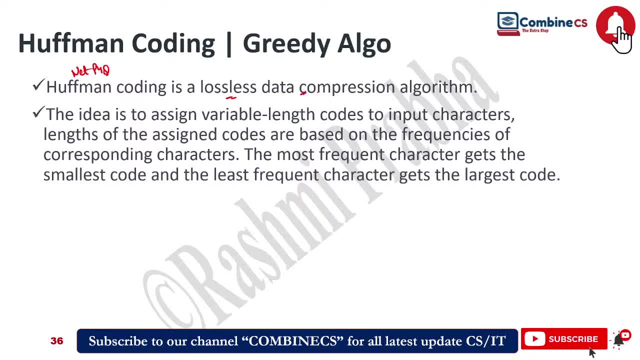 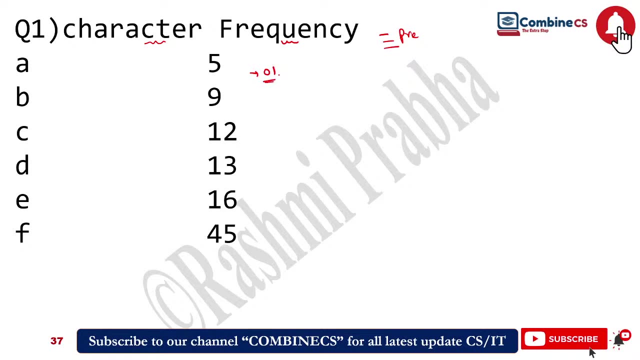 Is it for data compression or for data decompression? So you should know this. It is lossless data compression algorithm. Lossless means that when you convert any given characters, When you convert its frequency to 0,1 format, Then there will be no data loss. 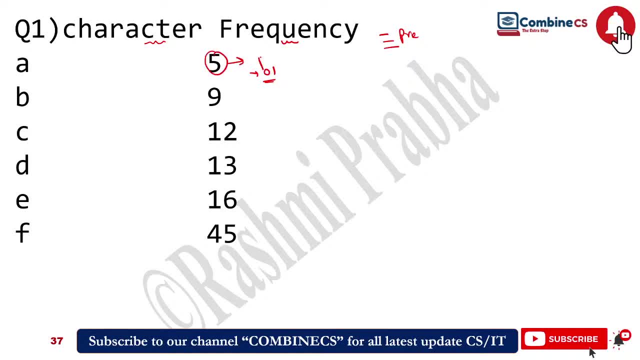 Because each and every frequency is transformed in the form of packets And whatever raw data is going in the packets, That is converted in the form of 0,1.. Correct, So whatever packet is transferred in the network, There should never be any packet loss. 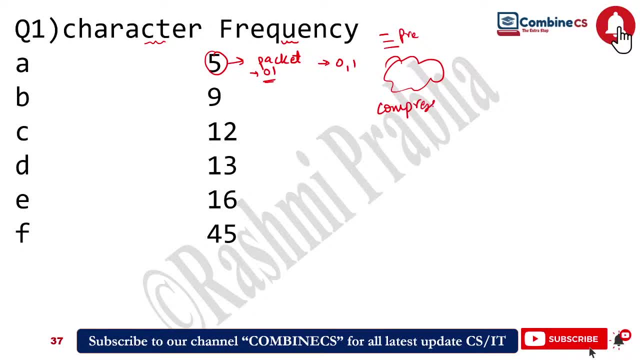 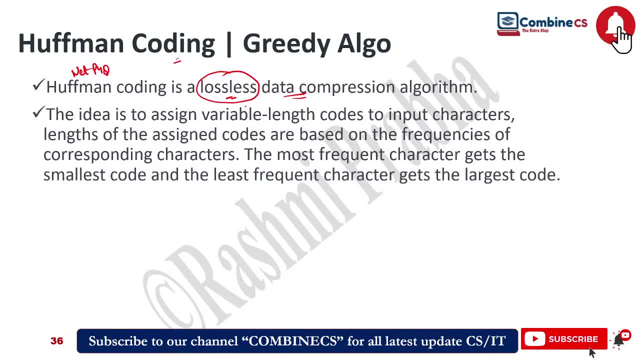 Why? Because, let us suppose, if you compress this file, Then sometimes our data gets lost in compressing. That is why we use halfman coding, Because here there is no data loss. This is a very important point. The first point: The idea is to assign variable length code to input characters. 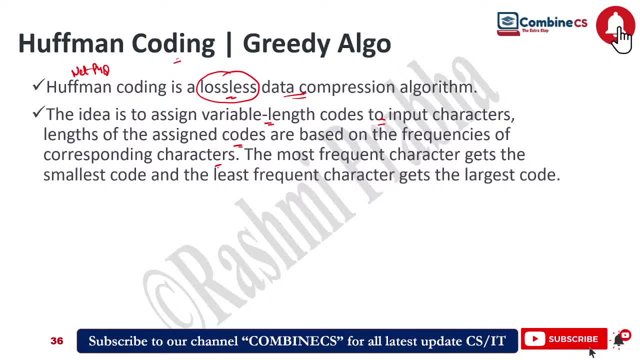 Length of assigned code are based on the frequency of corresponding characters. The most frequent character gets the smallest code And the least frequent character gets the largest code. So this is your statement. wise question. You have to understand this very carefully. If I make a tree like this: 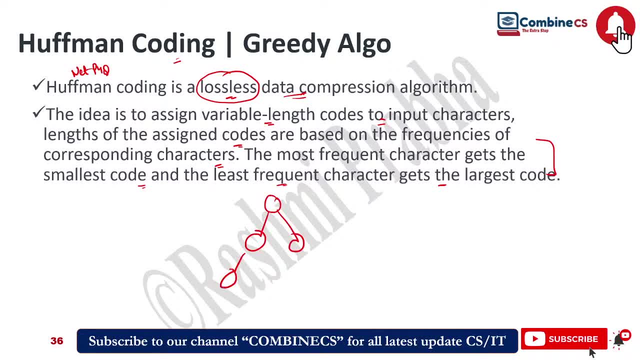 Okay, Basically, To make this tree, There will be a given frequency here. Let us suppose this is my tree. based on this frequency In this tree, What we have to do is We will randomly assign values of 0 and 1 in this way. 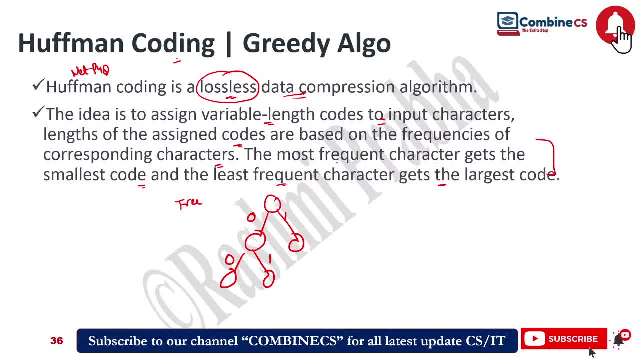 So here they have said this- The most frequent character- Let us suppose this node is A. Let me change the color. If you are watching this video, If you tell me The audio video is on A, B, C, D, E. 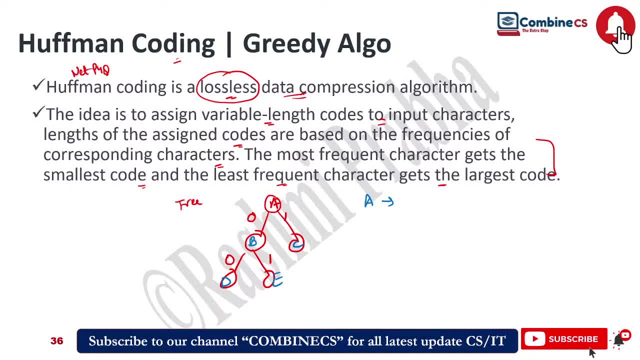 These are the nodes, Because there is nothing on A. So what will be the frequency of A Minimum value? If I talk about B, That is, how many nodes are you traversing? What is its weight? 0.. If I talk about D? 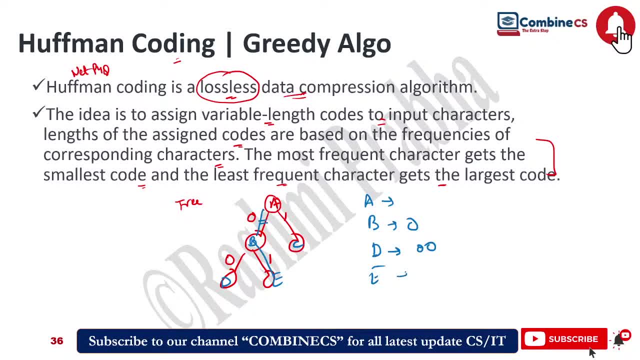 What will be the weight of D 0.. If I talk about E, What will be the weight of E 0. 1.. So what you have to understand here, You don't need to traverse here. That is why it will be least. 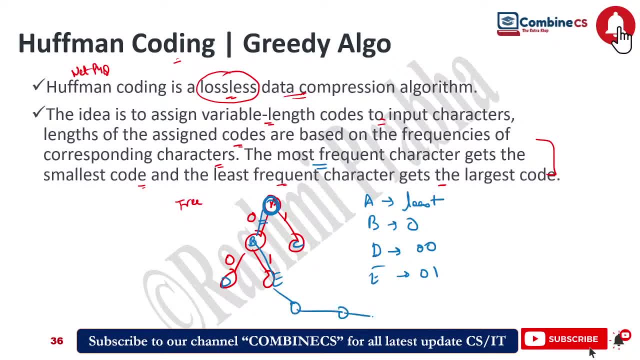 And the number of nodes. Let us suppose, If I make a diagram like this- The number of nodes- What will be its coding? It will be the largest code. This was your previous question, In which they changed the terms. Let us suppose. 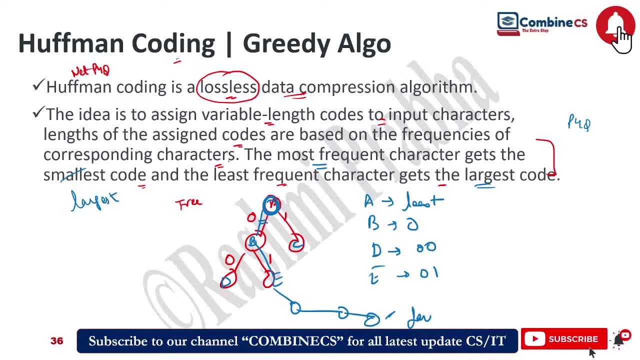 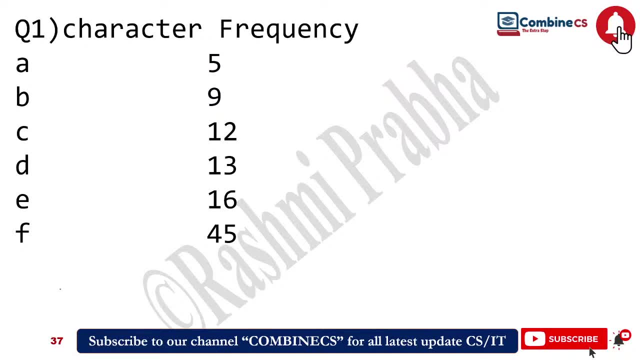 They will give the largest instead of smallest. You will have to understand What they are trying to tell you. This is the theory of half-mill code. Let us see What are the important questions And what kind of questions are asked in this topic. 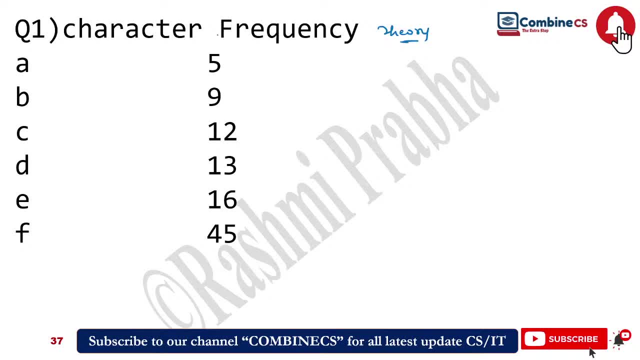 In the Jury. They will ask questions like What is the definition And what is the application, And you will be given a question like this in the exam, Which you will have to solve. How will you solve? I have not written the algorithm here. 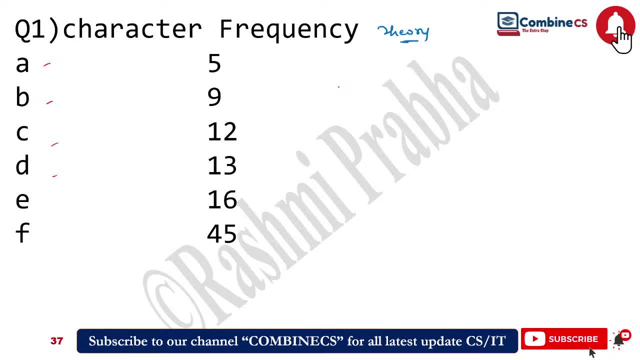 I will explain in a simple language How you solve this coding. You will have these given characters And you have to select two minimum values And then you have to add those two minimum values. After adding, you have to form a new node. 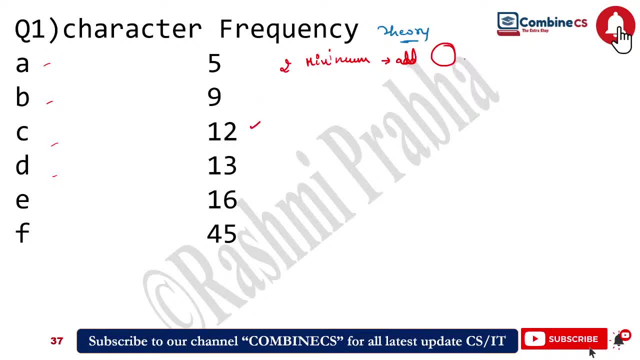 After that, you will take a third number, Then you will compare it with that third number And in this way, All the nodes will be made. That is basically. This is a question based on probability, In which, ultimately, What value you want, 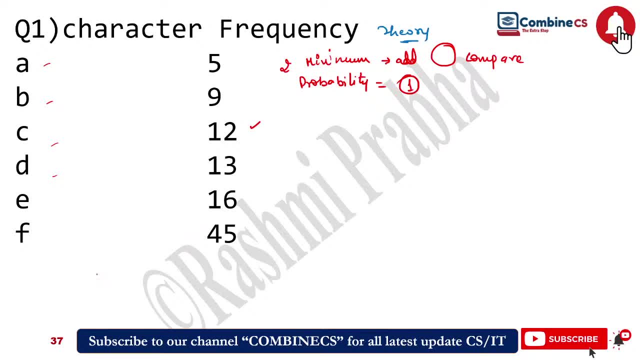 You want 1 value, Because we do not make the value of probability more than 1.. So the value of probability should be 1.. Let's start Now here. when you see this, This is the sorted. I have taken this sorted. 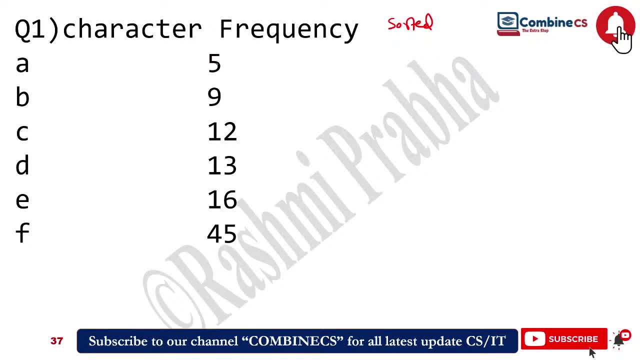 What can happen to you in the question? That it is unsorted. So the first step will be that you have to convert it to the shorted form, Because what do the learners do? They do not convert And they do not match the answer. 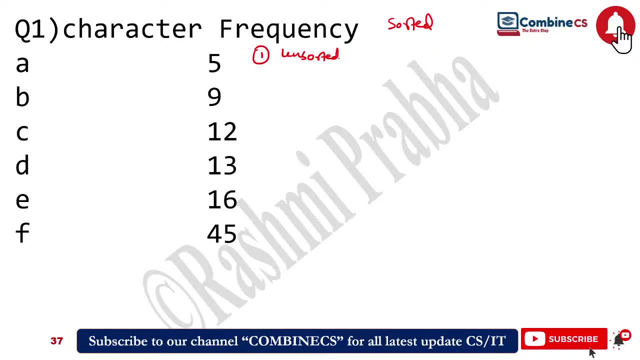 So first you have to be here. If you are unsorted, So you have to convert all the frequencies, You have to short. So here I have already written in the shorted form How to add. First of all, we will select the two smallest values. 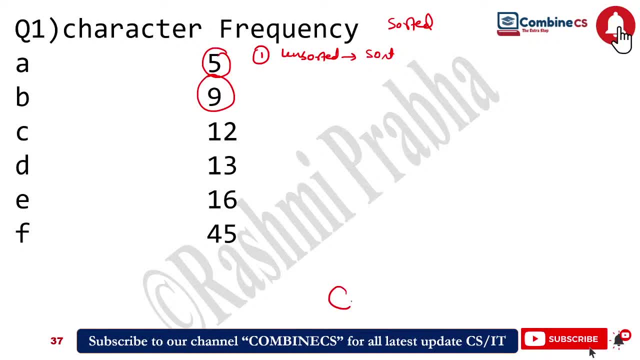 So what is the smallest value? 5 and 9.. So you have to write down in this way: This is b And this is 5.. This is 9.. Correct, By adding this, you have to make a new node. 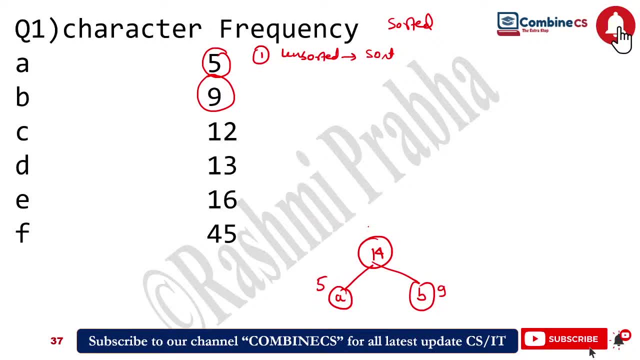 This will be 14.. 9 plus 5. That is 14.. Now what do you have to do? I have compared 12.. 12 is what It is less than 14.. What will we follow here? You have to follow the property of binary search tree. 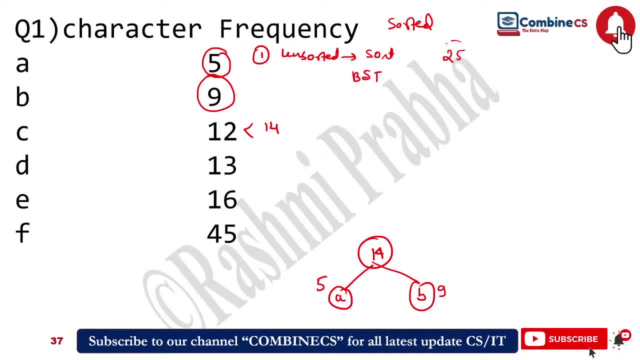 What is binary search tree? If your root node is, let us suppose, 25. Then on its left, Every node on its left will be less than 25.. And every node on its right will be greater than 26.. Correct, So if you follow the rule of binary search tree, 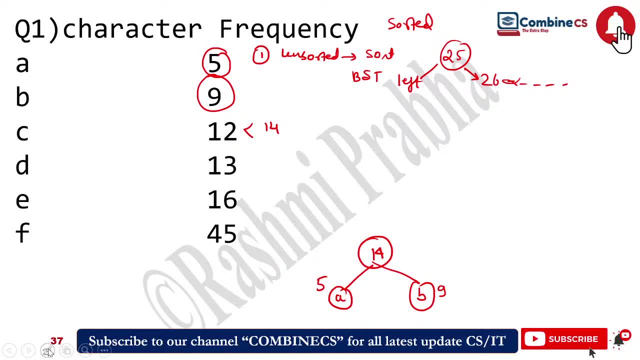 Then where do you have to insert 12? 12. You have to insert 12 here, That is on the left side. In this way, you will write 12 here And then you will add it here. I have explained you so far. 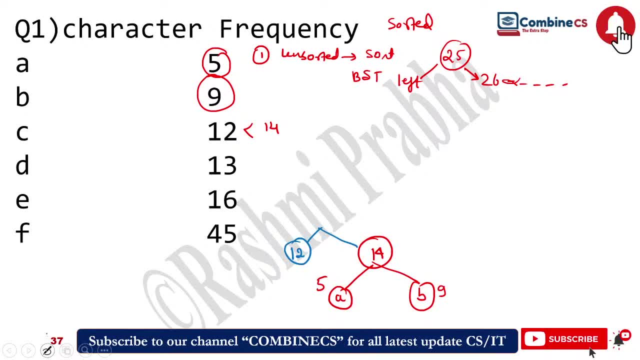 But there is a mistake here. What is the exception Here? you have to keep an exception in mind. Many learners have problems here. What is the exception here? Now you understand. here You have only compared one value. This is less than 14.. 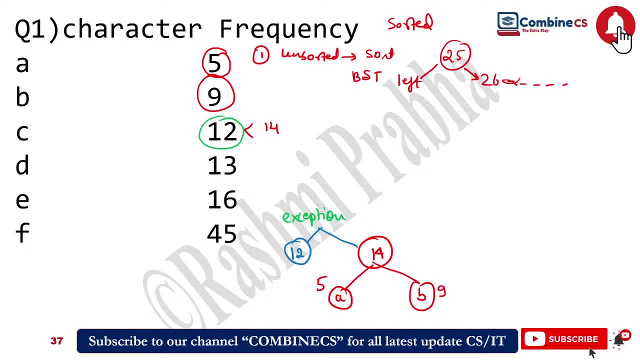 And you have added it here. What will be the value here? 26.. Correct, You have written 26 here. After that, you have taken the next value, 13.. Then 13 will come to the left. here You add these two. 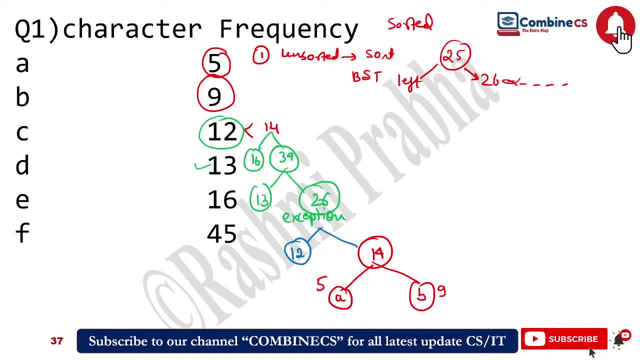 That is 9 and 3. 39.. After 39 there is 16 again. So write 16 here And add these two. That is 9, 6, 5 and 5. 55. And if you add 45 to the left of 55.. 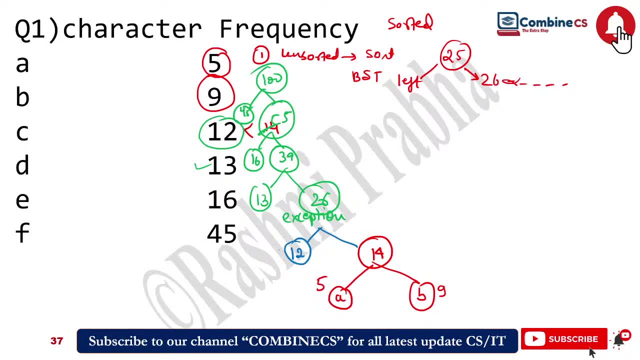 You will get 100.. You have to assign 0 and 1 here. Let us do this. This option will be wrong. This option will be wrong Because you have to understand this In the algorithm we have seen. first You have to short the list. 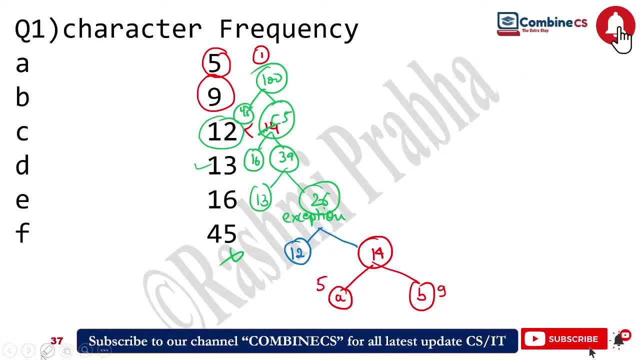 After that, add one more element. So when you add two elements And you are getting 40.. The smallest is here, 5 and 9.. When you add this, You will get 40.. Correct, How many values are less than 14, so what you get here is 2 values are less. 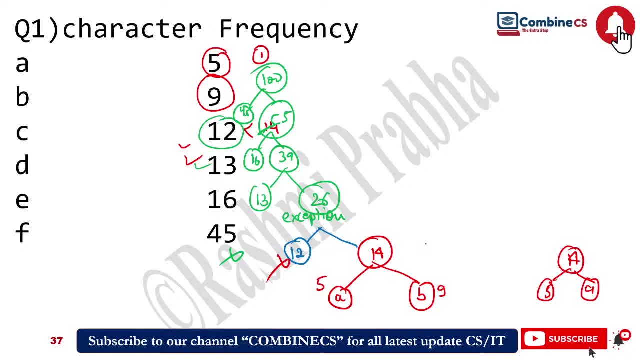 You will not take only single 12 here. What you have to do here, because all these are in one level. You have to write 12 here, you have to write 30 here And you have to add this 12 and 13.. 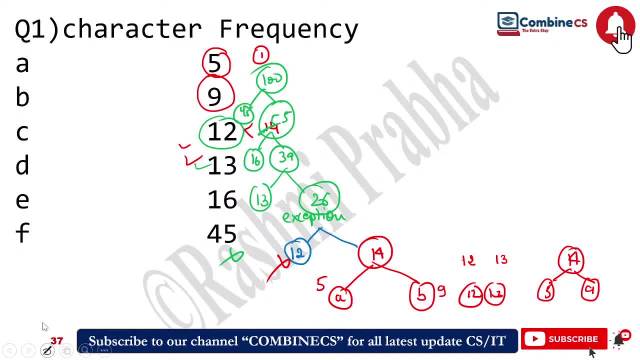 When you add this 12 and 13,, then what you will get? You will get 5 and 2. 25.. Correct, So we took these two values. After that, you got 16.. Now tell me, with whom will you add 16?? 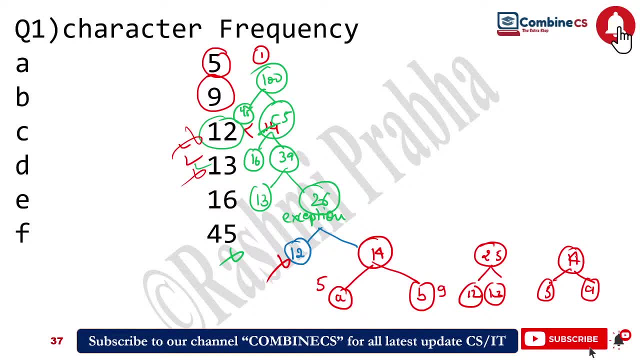 Will you add with this or with this? You can see here that 16 is greater than 14.. It is smaller than 25.. But because we already have 14 as an element, you will add 16 in 14.. And how you have to write? 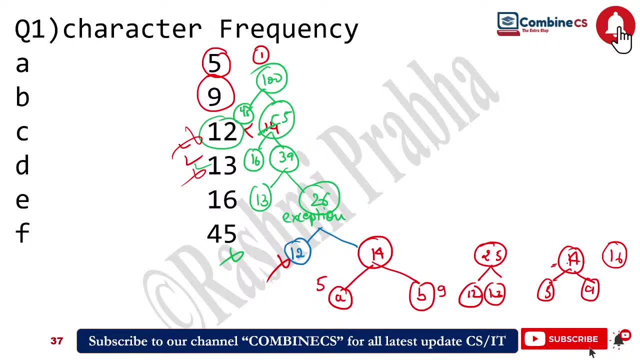 Because if your binary set is a property of all the colors, then it should come to the right. So you will add 14 and 16 in this way. So what you will get? You will get 0 and 30. Correct. 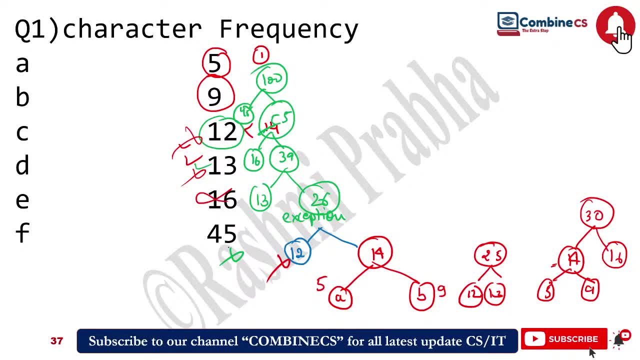 You got these two, So you have solved till here. Now it is your turn, 45. So where will 45 come? So these 25 will be added in this way And you will get 55.. And you got 55 here. 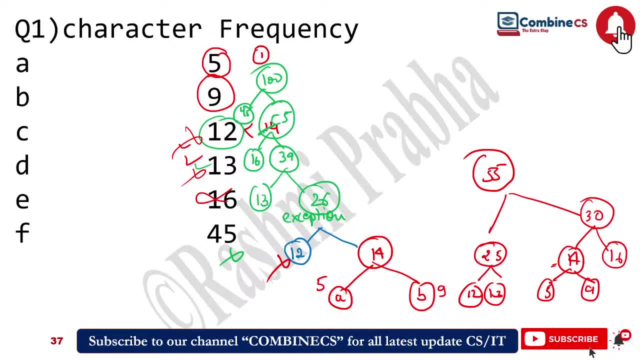 Before this, because here before 45, you have 25 also. This 25 will also come. So here 25 and 30 will be added, And then you will quote here 45. And in this way 45 will be added. 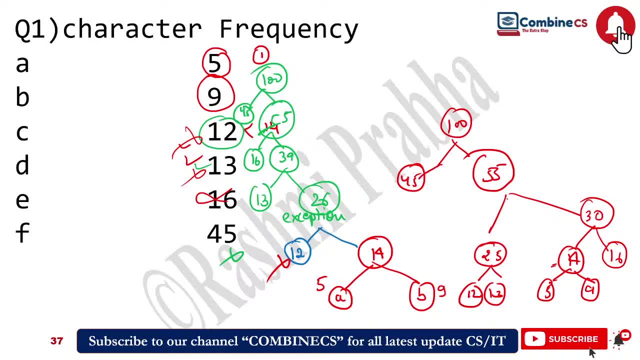 Then it will be 100.. Actually, you will get this 100. But this is the correct way to solve this question. And after that, what you have to do, You have to assign weight. So how will you assign weight? That is, you will start assigning it 01.. 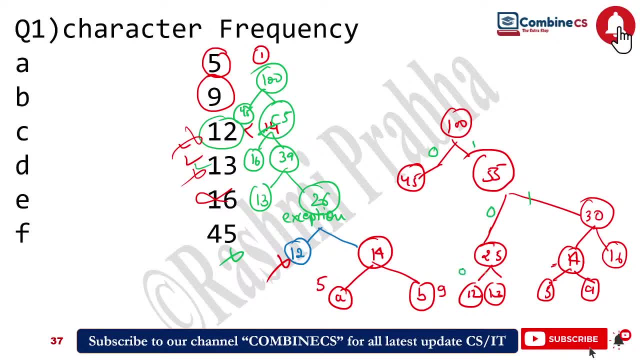 In this way, you have to assign 01, 01, 01 for each age, And then you have to write its frequency. Let us suppose, if I talk about A, This is A, This is B, This is C, This is D. 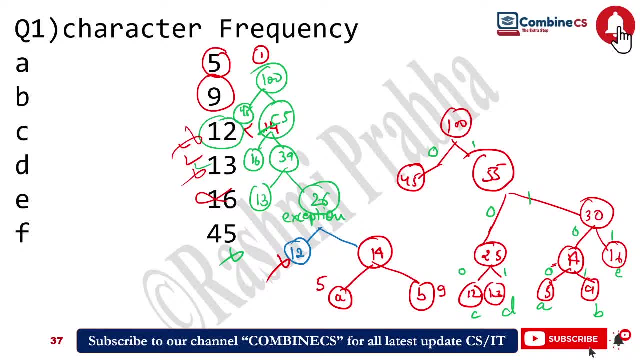 And this is E And this is F Correct. If someone will ask you the frequency of A, what will happen to the frequency of A? You have to put down all the values here. After that, what values are you getting? That is: 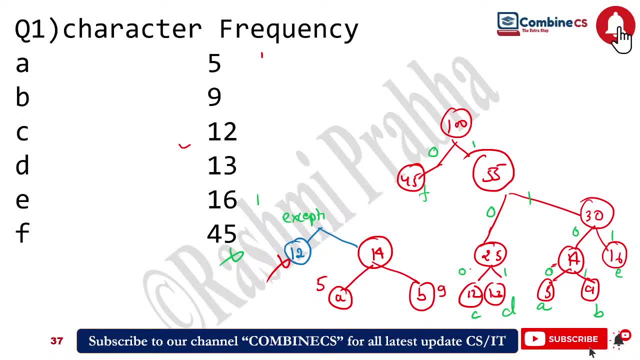 A is here. What will be the value of A? You will start from here: 1100. 1100.. In the same way, what will be the value of B? 1101. 1101. 1101.. 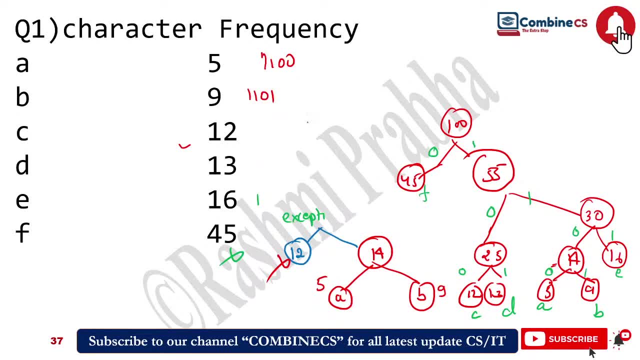 In this way, you have to get the frequency Here. I would like to pay attention to one more important point Here. I would like to pay attention to one more important point Here. I would like to pay attention to one more important point. 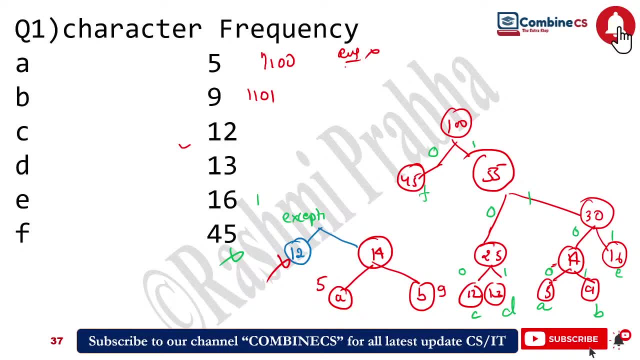 Sometimes the answer will not match. In that case, what will you do? It is a rule that you assign 0 and 1 in this way, But if you never get the answer- Because this is frequently the case- in the gate? 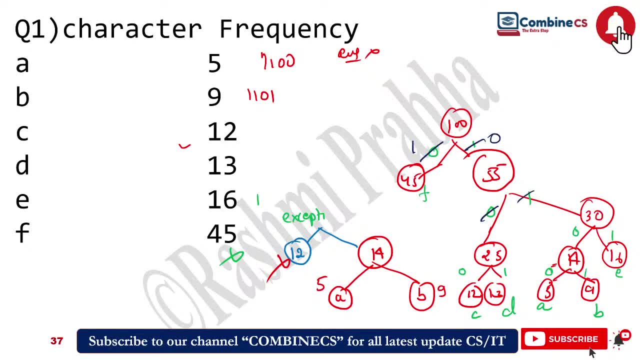 So you can take it 1 and 0 instead of 0.. Considering this, you can check to match the answer In the answer. it is possible that it can also be considered in this way. You just have to change its position. 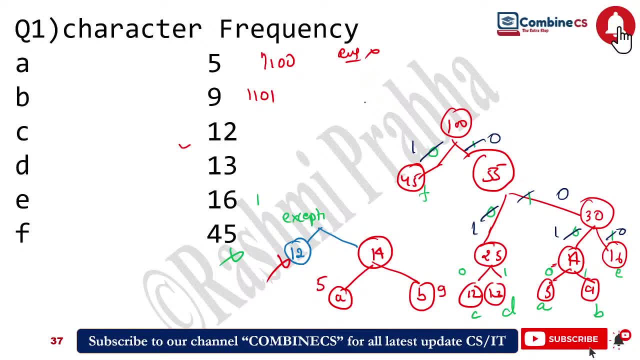 And you can solve it this way, And you can solve it this way. So, basically, what did we do? We gave the frequency according to this corrective. We gave the frequency according to this corrective. half-man coding: It means that we have compressed in this form, So this is known as half-man. 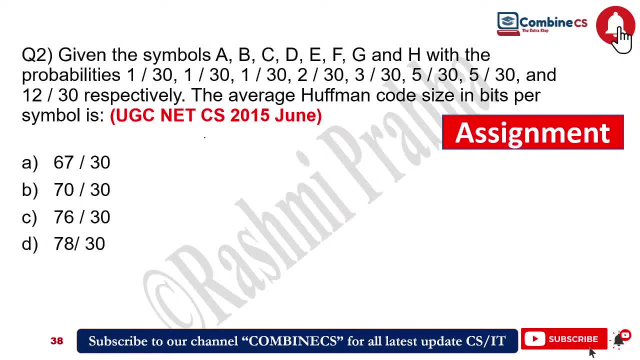 coding. Now we will see some more important questions. Before that, I would like to tell you how frequently this question has been asked And you can see in UGC date, 2015, this question has been asked. So whoever is watching this video, they need to solve this question. 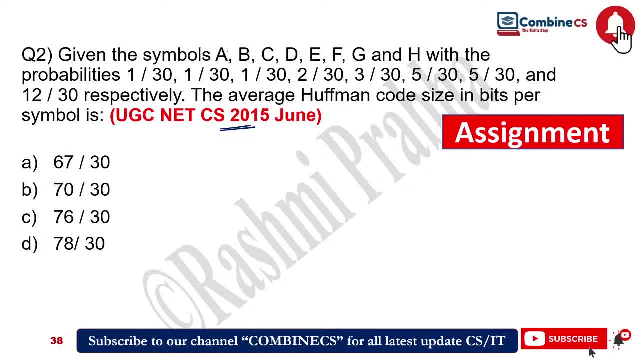 and tell me the answer in the comment section Here the question will be given in the same way. A, B, C, D, E, F, G, H. These are the symbols. You have given these symbols here And you have given the probability of these symbols And, respectively, Respectively means: 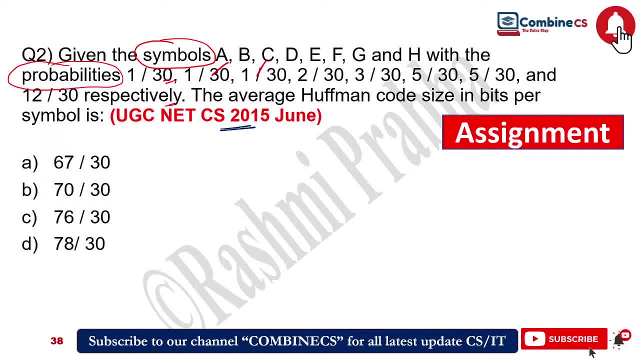 that the value of A is 1 by 30. You have to execute the value of B in this way in the sequence. You have to find the average code size in bits per symbol. You have to know the average size. So how do you know the average size? Let's suppose this is the code size in bits. 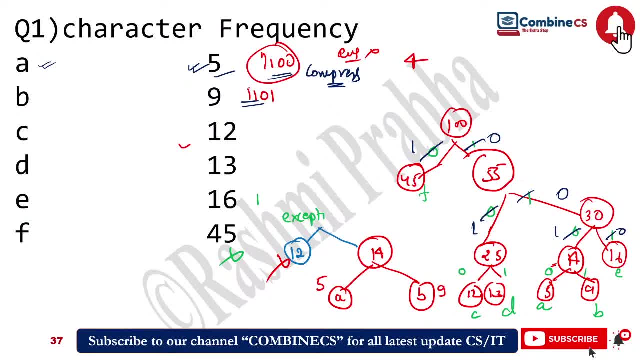 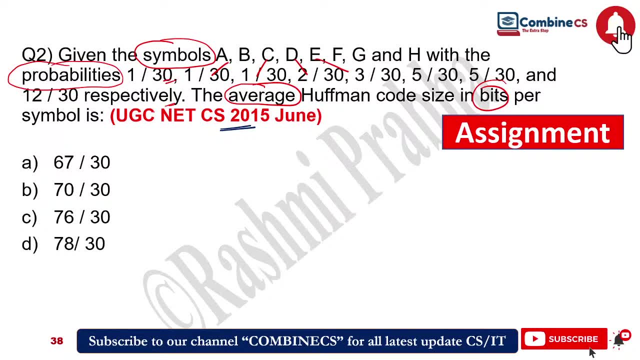 per symbol. You have to know the average size. So how do you know the average size? Its average size is 4.. Its average size will also be 4.. So you have to count the number of bits as per the number of bits. How will you solve this question? To solve this question. 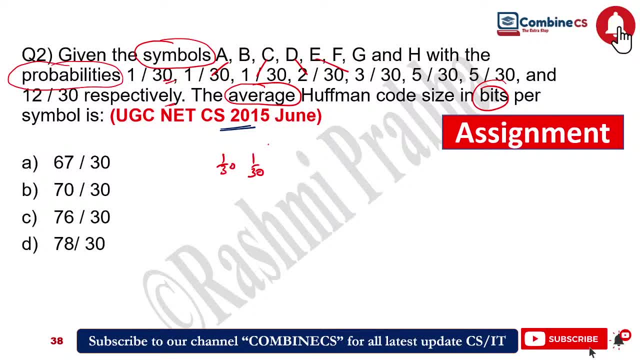 you have to use either 1 by 30 or 1 by 30. Otherwise you can take it in the point And let us suppose, if I talk about the point, you will get 33.. Correct, So let us suppose you get 33.. So now you have to add these decimal numbers in the same way You have. 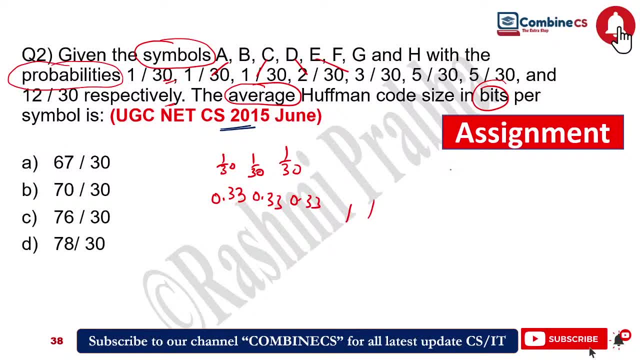 to add these decimal numbers in the same way And in the comment section. you have to provide me the answer for this question. If it is not solved, you can tell me in the comment section of this video. I will solve this question tomorrow. Okay Now. this is again the previous. 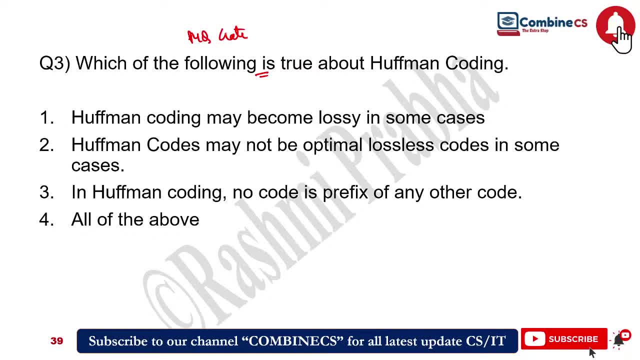 year question of GATE. That's why I explain the previous year question with the concept in every video. Which of the following is true about the half-min code? So whoever is watching the learners video quickly provide me the answer for this. They have been asked. 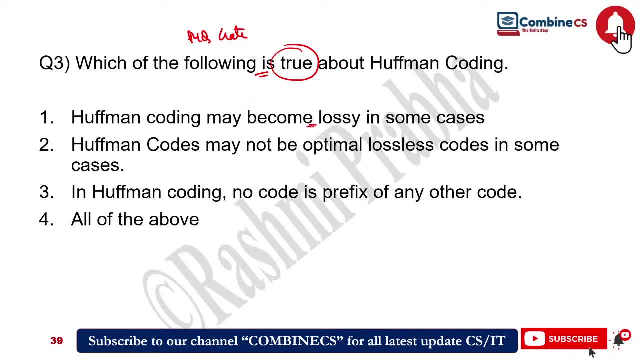 if true, Half-min coding may become lossy in some case. Lossy, sorry, Half-min code may not be optimal Lossless code. In half-min coding, no code is prefix of any other code. all of the above, Which is true statement Now we have seen in the starting of the class: 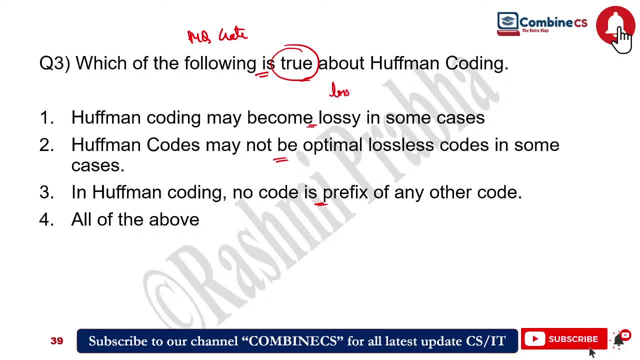 that half-min coding is usually used because it gives you lossless data. Correct, So this statement is false. After that here they have written: may not be. May not be means there will be lossy, otherwise it will be lossless. This statement is again false, Sorry. So if 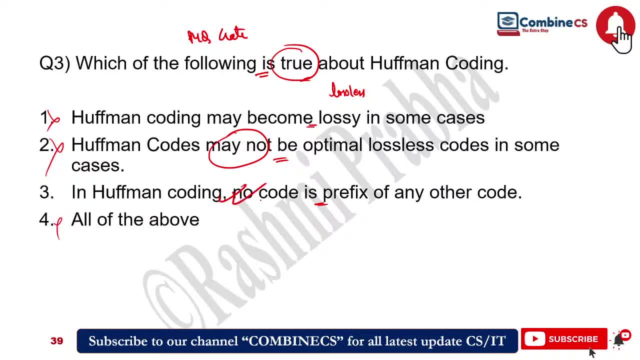 this is false, then this will be false. Hence this is the correct answer. So here the prefix which you are representing in the format of bits For every character. here your prefix will never be same, It will always be different. No code is prefix of any other code means. 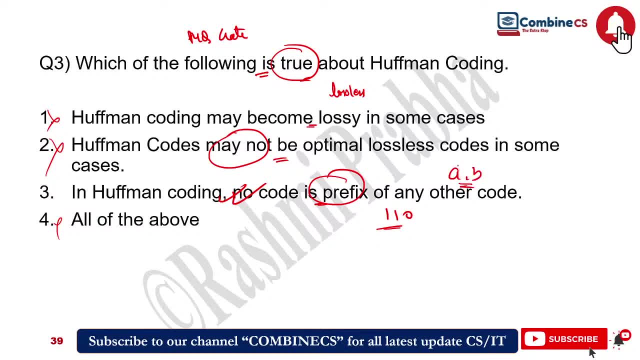 that the value of any two character will never be same. Okay, This is how you need to solve the question. You need to know both theory and practical. Good evening, I guess audio and video is proper. So whoever is watching, If you want to tell me No? So this is the. 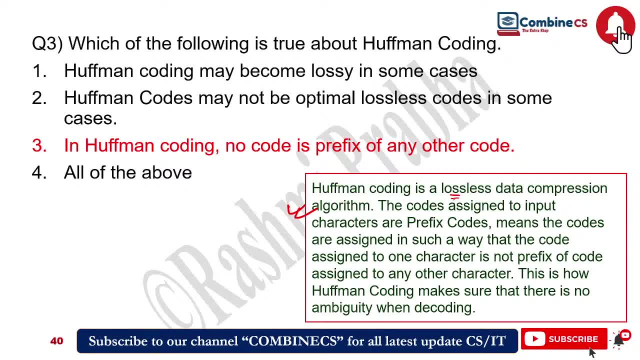 answer and this is the explanation. You can read it: Half-min coding is a lossless data compression algorithm. The code assigned to input character of prefix code means the code are assigned in such a way that the code assigned to one character is not prefix of code assigned. 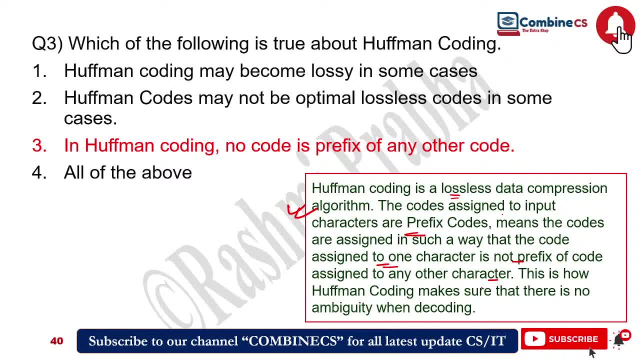 to another character. Don't get me wrong. It is not prefix of code assigned to another character. This is what I just told you. This is how half-min coding makes sure that there is no ambiguity when coding. So watch the videos very carefully, because the daily 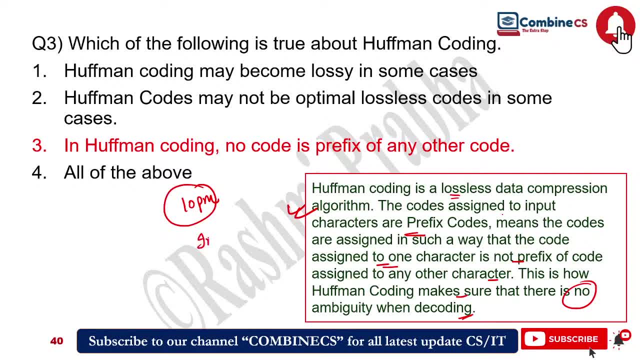 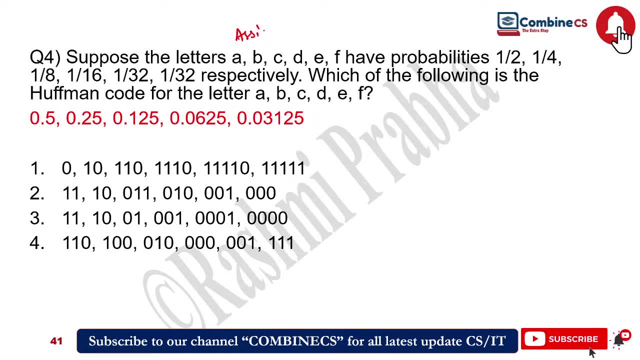 10 PM video is happening In that I am trying to tell you the concept of whatever is your important topic, Because in UGC net you are already being asked such questions and along with that you have to do the previous year questions. So this is again assignment to. 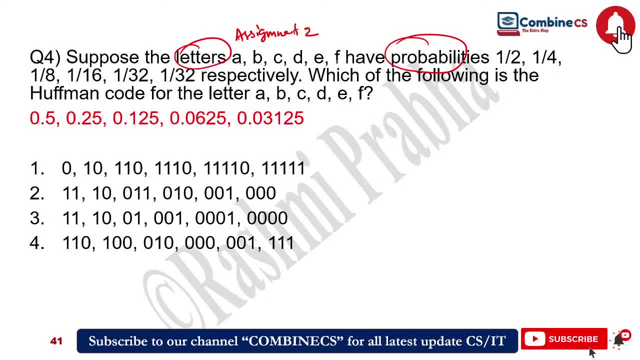 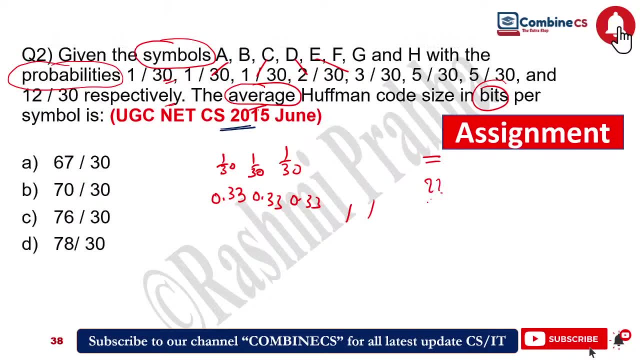 you. These are the letters given. This is the probabilities given. here You have to tell, which are the following: is the half-min code for the letter. In any question they will ask you in this way: what is the average value? So, in average value, basically you have: 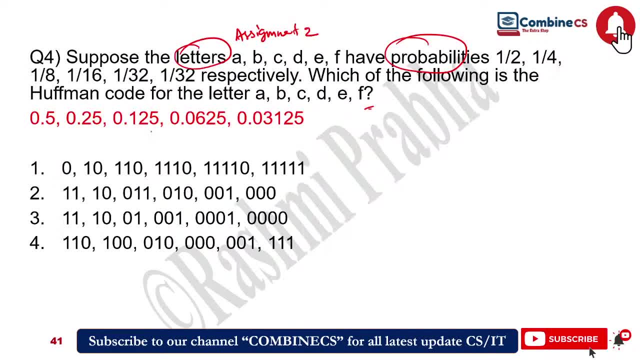 to write by multiplying with the characters, And either they can give you the sequence. So this sequence means that you have to make its full tree structure And after the tree structure you will write 0101 for each character, for each letter, And then you will write the. 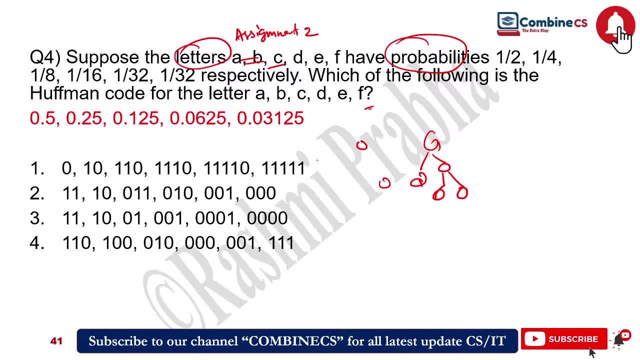 value of each character here. So in this question which I have discussed in the previous question, Let us suppose if you have taken this 01.. If the answer will not match, then what you will do is you will replace 0 with 1. Then you will try. So I have given two questions as an assignment. 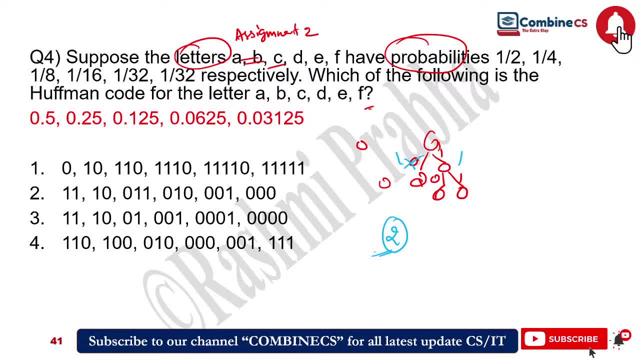 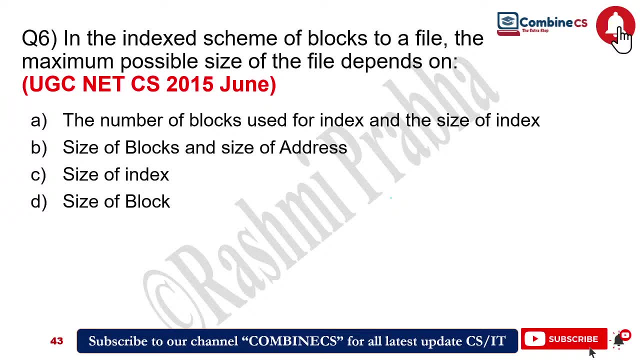 you have to do, And if there is any doubt then you can ask me in the comment section. Thank you so much. Now let us start with our previous year question. Quickly provide me the answer in the comment section. Today we have 11 questions to go. This is question number 6.. 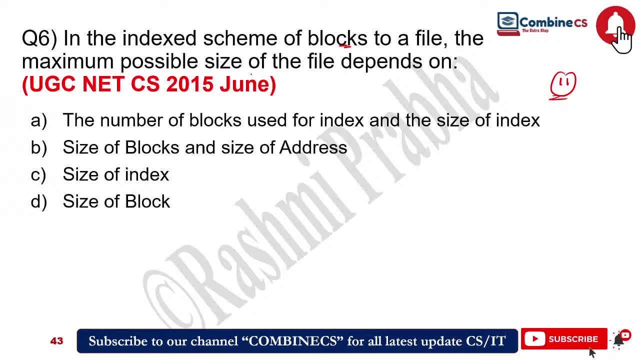 In the indexed scheme of block to a file. the maximum possible size of the file depends on what Already we have covered indexing in the playlist of DBMS database management And, if you will see, in the crash course also I have talked about the indexing of Unix file. 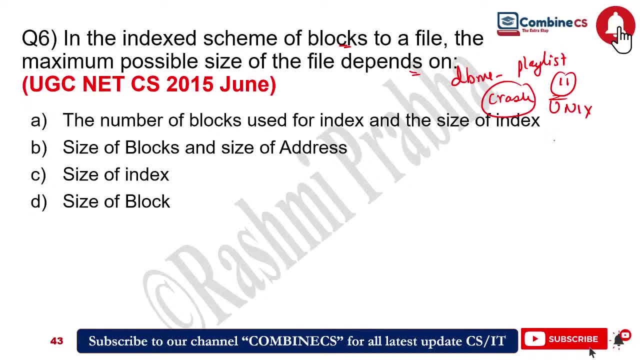 system. So you must watch that video, Because your operating system, whether it is Windows or Linux, your concept, does not change Correct. So what will be the answer? When you will make an index file, then what will be stored in your file system, in the index? 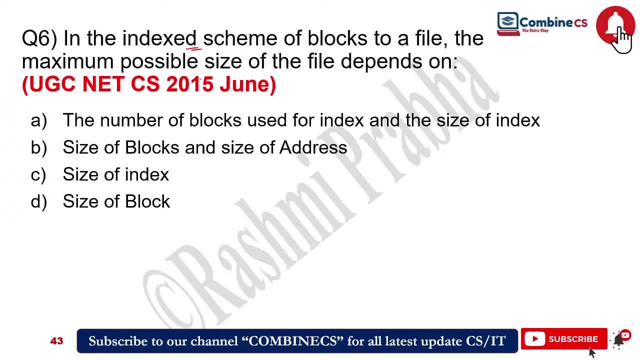 scheme. What will be the maximum possible size of block to a file Depends on which The number of blocks used for index and the size of index. size of block and size of address. size of index or size of block. What will be the answer? Just tell me in the comment section. 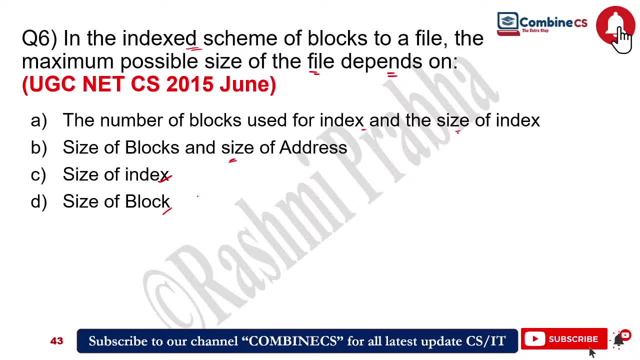 So let us see the answer. The answer will be option 1.. I have told you in the last time also, when you use the index scheme, then you have to tell the number of blocks there and along with that you have to tell the size of it. 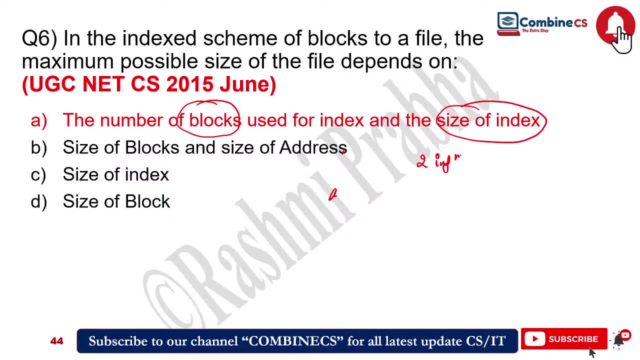 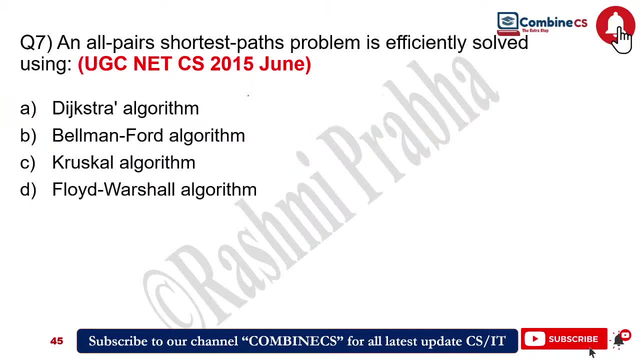 Correct. So these are the two information which are stored in your index scheme Already. this has been asked in your previous questions in UGCNet in 2016.. Now question number 7.. And all pair shortage path problem is efficiently solved using which algorithm? 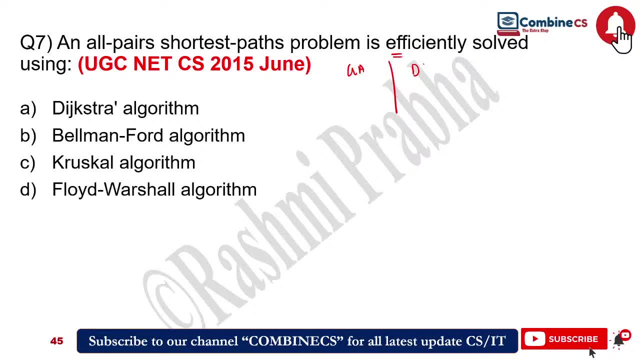 I had told you yesterday also that you have a greedy algorithm: Divide and conquer dynamic programming. you should have a chart of all these so that you can easily reply to such questions, because these are the theory questions and always you will get one question in every competitive examinations. 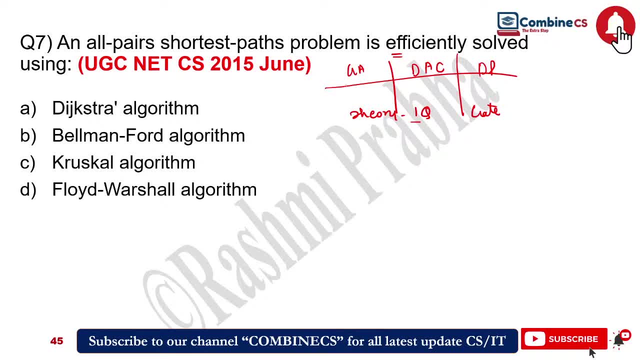 Either get or not get, So you can easily solve all pair shortage path problem, Like Castro, Bellman-Ford, Kruschikl or Flood version. So let us see the answer. The answer will be Flood version Correct, Because in all pair shortage path problem you have to consider all the pairs here. 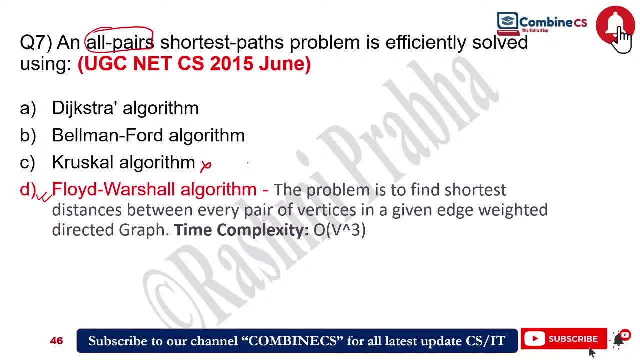 If we talk about Kruschikl, then Kruschikl is basically used for minimum spanning tree. So here, if you include only that edge, then it will take you to the minimum cost. So in this way, if you are solving a portion, then you must know the properties of other options as well. 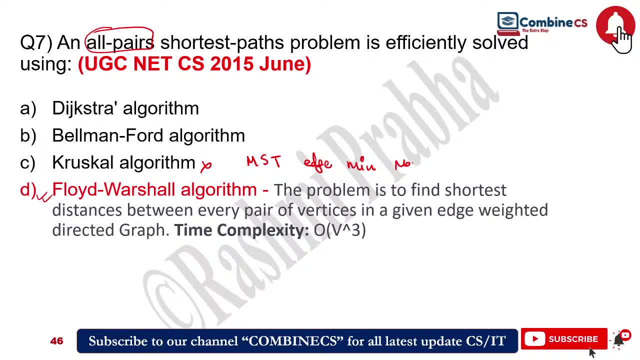 The algorithm has also asked you a question in 2020.. So it is not necessary that always. they will give you a graph and they will ask you: what is the minimum spanning tree? They can ask you the question based on concept as well, Correct? 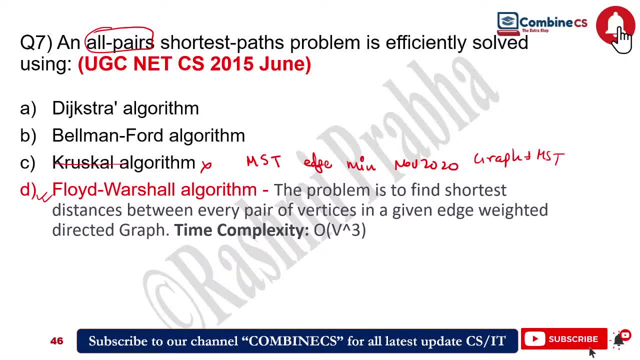 So this is the minimum spanning tree, so these options will be cut here. If we talk about Bellman-Ford and DeCastro algorithm, So basically in DeCastro algorithm also, you select the path which is your shortest, Correct. 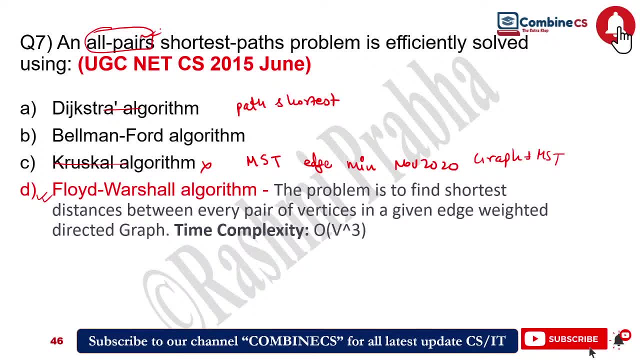 Here we consider all pairs path Correct. We don't do this Now. if we talk about Bellman-Ford, then in Bellman-Ford we don't talk about all pairs shortest path. We do this in Floor Washer because this problem is to find shortest distance between every pair of vertices in a given edge. weighted directed graph. 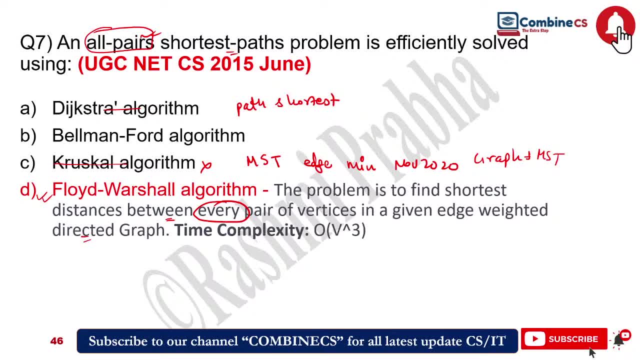 And here, when you draw any graph, it should be directed and weighted Means. if you have a graph like this, then how will you find out the path shortest? It must be assigned some values, Correct. So what is this? This is known as directed. 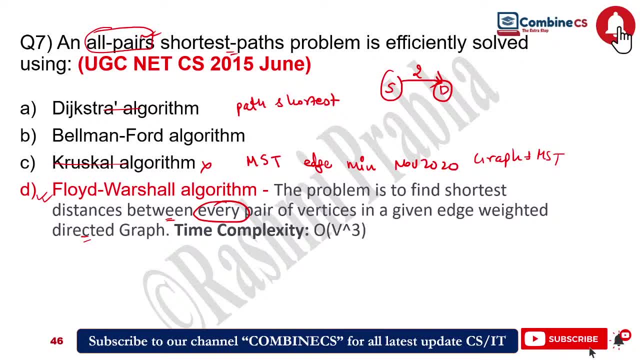 You are telling direction, this is the source, this is the destination And the value you have assigned here. this is known as weight. This is known as weighted directed graph. Now in UGCnet, once in the previous year question you were asked about this in properties. 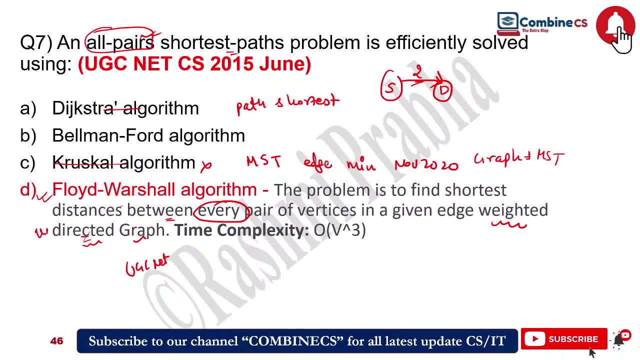 What will they do Here? they will write undirected. So always keep in mind that all your algorithms are correct. Okay, You don't talk about direction in Cushical and Prim's, But if you use D'Castro algorithm or travelling salesman problem or Floor Washer algorithm, 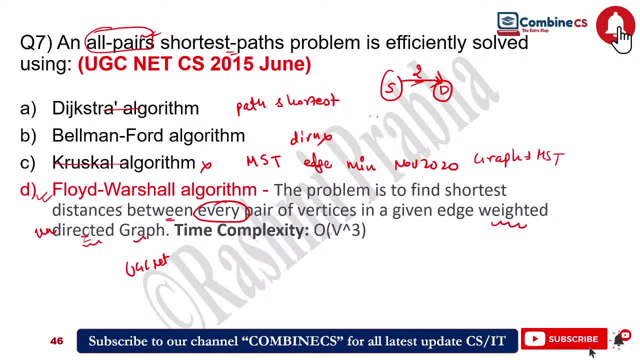 you will have to give direction compulsory. You are given in the question that you have to reach this destination and this is the start node. So which route will you take? Directed graph will be compulsory there And again. if you are doing all these algorithms, then you must learn the time complexity. 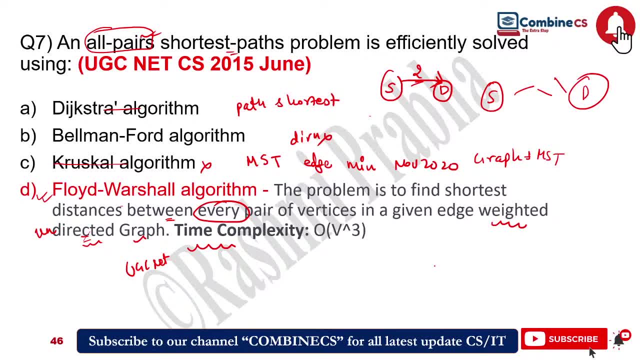 You must learn the time complexity. So in yesterday's video we have covered all the shorting searching. So if you haven't seen that video yet, just go and watch the playlist of crash course. It has all the important videos covered. And if you like the videos, then do subscribe to the channel and share it with your friends as much as possible. 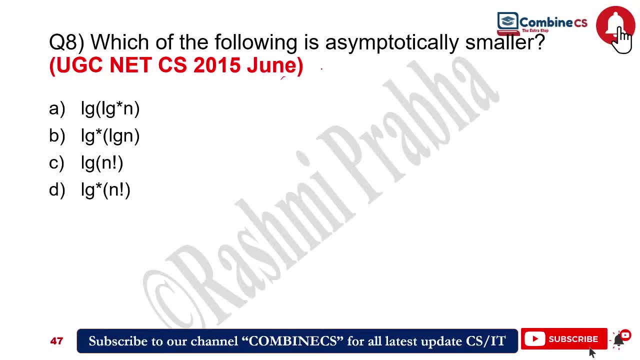 Now this is again. I am just giving you the idea that which equations you have to prepare for the examinations. Which of the following is an asymptotically smaller? Which of these four options will be smaller? Simply, you have to learn a chart. 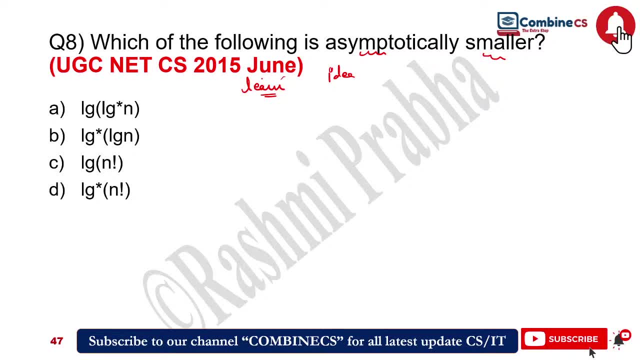 You can solve these questions by chatting to BC Swap. So what will be the answer? Thank you so much. What will be the answer for this question? You must know the hierarchy to learn the algorithm complexity. So let us see the answer. What will be the answer? 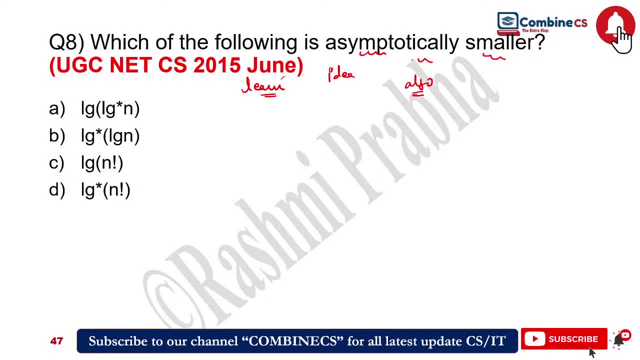 Whatever you have learnt, tell me once Those who are watching. I guess only one member is replying. What is the rest doing? If the rest is replying, then yes or no, Whether you know. if you don't know, then write a pass. 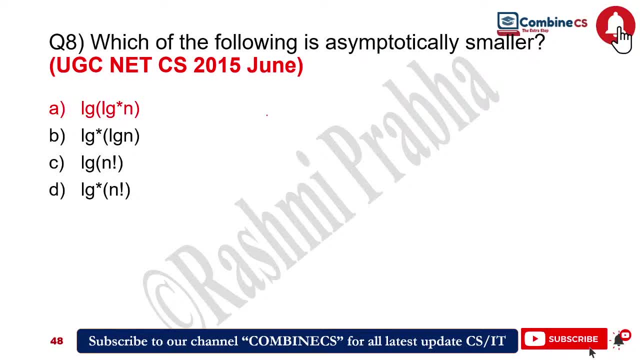 So that I will just tell you the answer. So let's talk about smaller here. What will be smaller? Always remember, the factorial will always give you a greater value. The most greater value will be given by the factorial. Correct The thing is, when you put a log here, then obviously the value will be reduced. 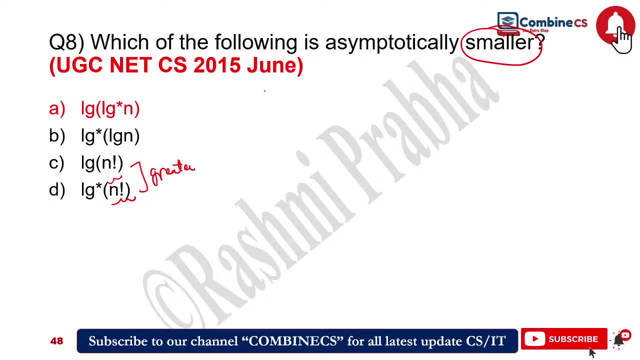 So here every statement has a log. So we don't know that when you solve any algorithm, if it is being executed at n number of times, if you put a log in it, then what will happen? It will be a smaller value. 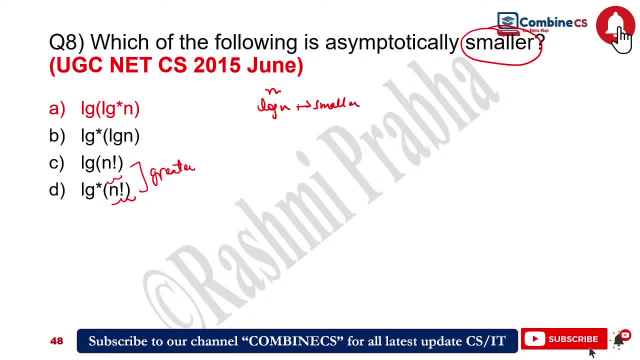 Correct. It is a smaller value. So, simply, if you knew the concept of just these two, then you can easily eliminate it. Smaller is asked. Smaller will be option 1. Because here a log has been put. It is the value of a star. 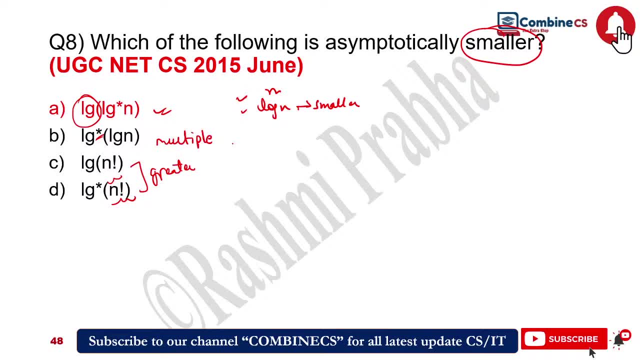 It means that it has gone somewhere in your multiple. Multiple means you can also call it exponential, So hence here your answer will be A as a smaller. So whoever is watching this video, tell me the letter in it Which has greater complexity. 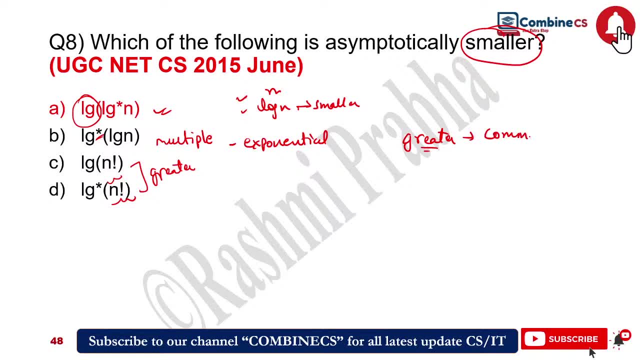 Or you can do one thing. You can write me an answer in the comment section. What is the greatest complexity When you run any algorithm? suppose if it is a chart complexity, then what will take the greatest time? Tell me in the comment section once. 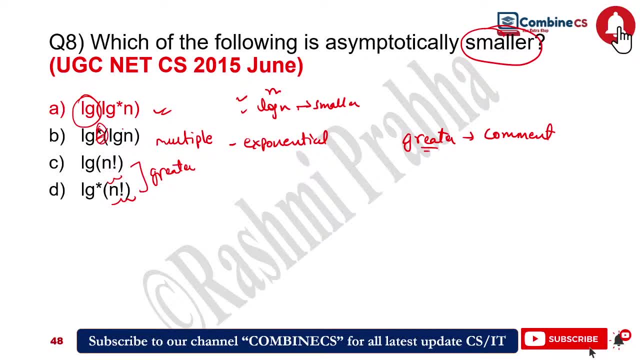 No, if you see this multiple symbol anywhere, I am just explaining. If you see a multiple symbol anywhere, it is just the multiplication. This is how you do not get confused, Because answers will get confusion in this way, Because what you could do is: 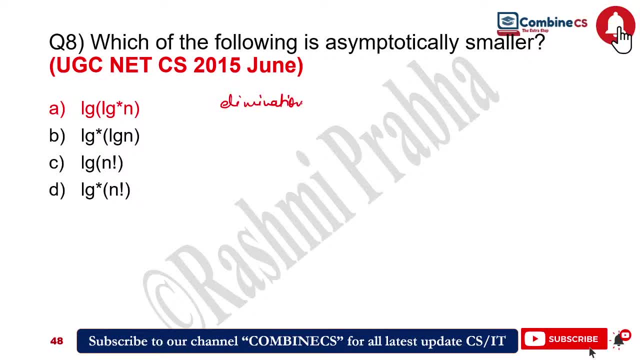 you could solve it with elimination method. How will you solve elimination method? If you have asked smaller, then you have to cancel factorial first. After canceling factorial, you understand that here is a log star and here is a log n. So here we want that log n is smaller than n. 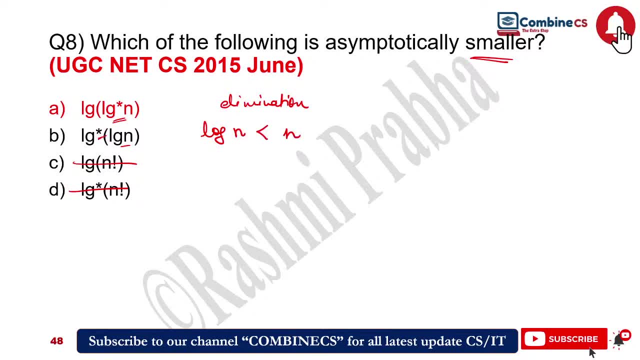 Correct This much. we were clear Now here. if it is a matter of a star, then you understand a simple thing: If at any n, if you add a star at any n, or if you understand power, then what will be the power? 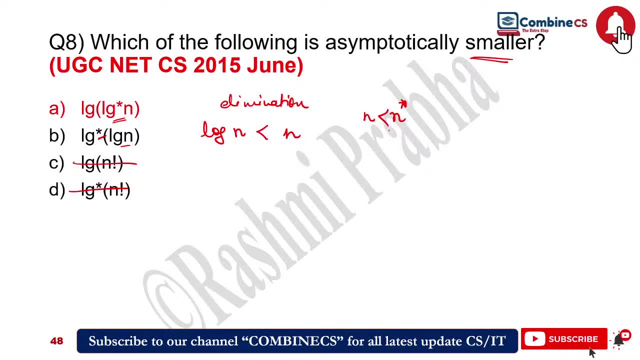 It will always be greater value than n. Its value will always be greater. So, whether it is a log or anything else, this is a simple log And this is log star. So obviously this will make its value a little higher. So that is why option A is the correct statement. 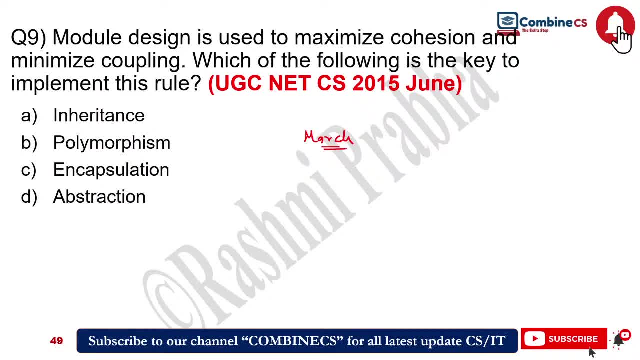 Yes, this is March. Almost March is completed. I am just telling again and again that you have 30 days time limit. You have to make a target And you have to start revision from now For May 2021. examinations for UGCnet aspirants. 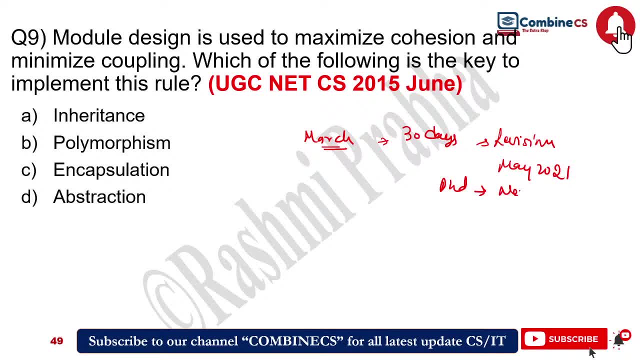 And those who have PhD examinations in next week, that I know that there are examinations in next week of Mumbai University, So this video is so helpful for them too. If you feel that you have any doubt on this topic, then you can write that too in the comment section. 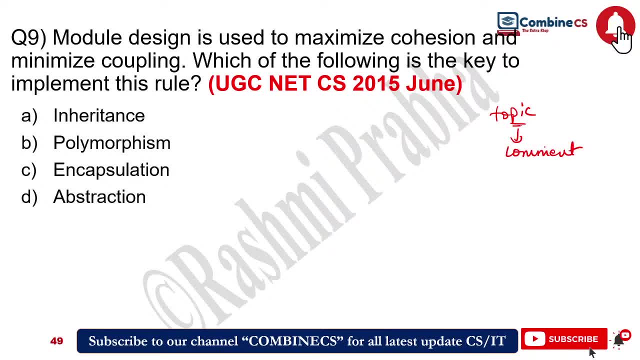 Because if you give me feedback in the comment section, then it is possible that on the basis of your feedback, I will complete the next video on the basis of your demand. Now, if there is a greater here, let's suppose if there is a greater question here, 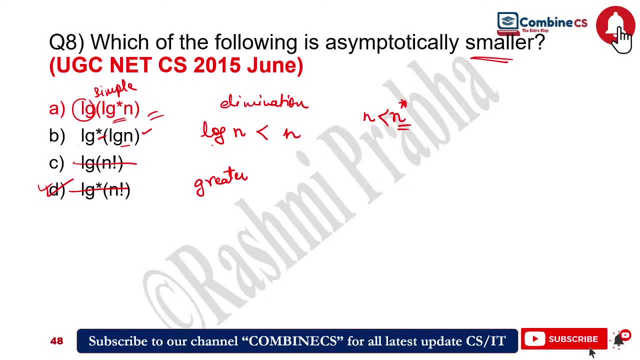 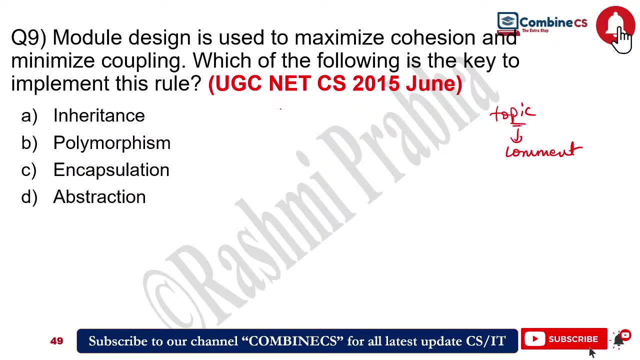 then option will be option D. If there is a greater question in the same question, then option B will be the answer. Now, question number 9.. Very important question, Very important question, Which I have taken from software engineering. Now I am just giving you another type of question. 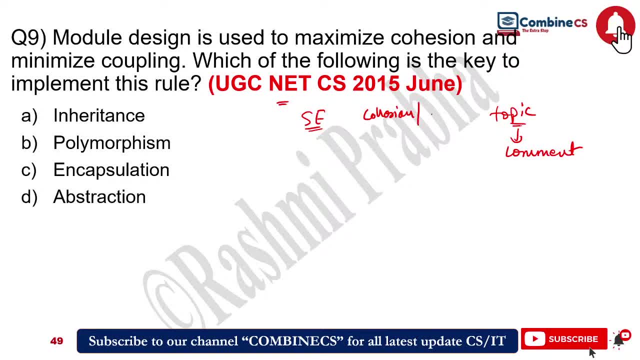 That I have already provided a trick of cohesion and coupling. If you have not seen that video, then you should definitely check it on the channel. And apart from cohesion and coupling, you are also asked this kind of concept based questions from software designing. 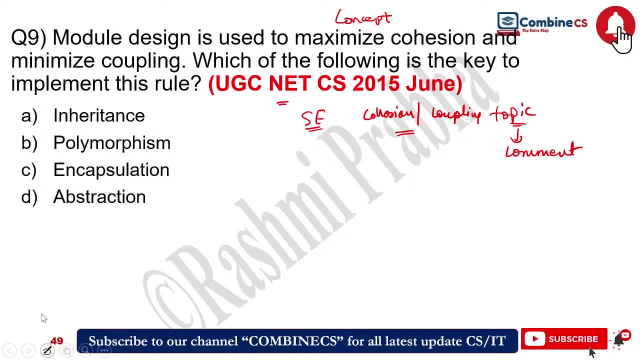 Correct. So what will be the answer? You can easily relate that here you should know the concept of object-related programming and you should also know the concept of software engineering. Let us see. The answer will be encapsulation. Basically, if I eliminate here. 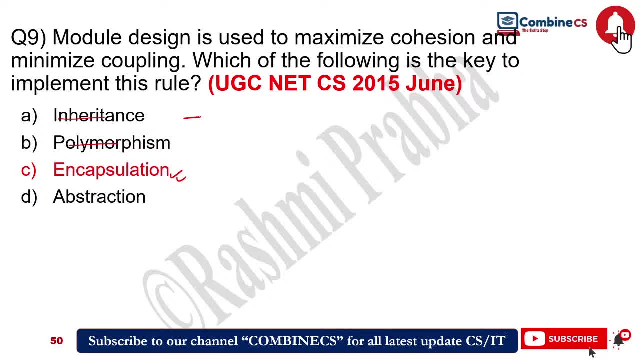 then inheritance polymorphism will not happen. Why? Because if it is about inheritance polymorphism anywhere, then you can easily solve this question with the relationship of parent and child here. But because they have said here that module design is used to maximize cohesion and minimize coupling. 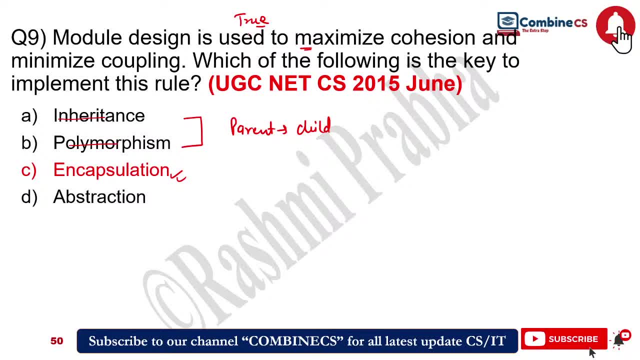 So this is a true statement. First, you have to understand why, Because this type of question will ask you in true and false. So this is a true statement. Now they have asked which of the following is the key to implement this rule. 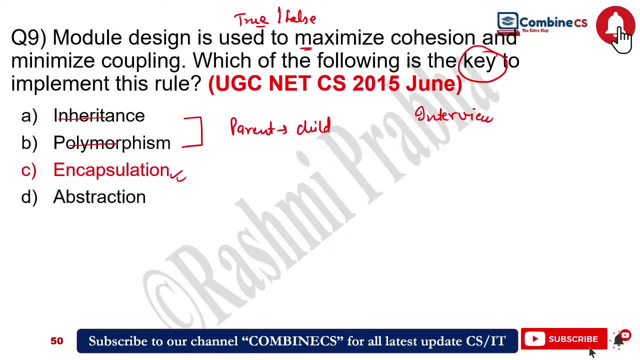 Now this has become your interview question. In interview question, when you go for the claim or, as a fresher, when you go for the interview. they will never ask you what is inheritance, what is polymorphism? No, They are going to ask you. 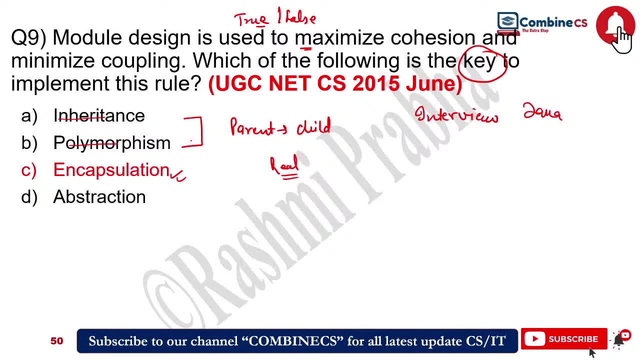 for example, how can you explain inheritance property? What will you say? Parent-child relationship? It is about encapsulation. What will we do in encapsulation? Let us suppose this is a class. In this class, what will you do? Data and method. 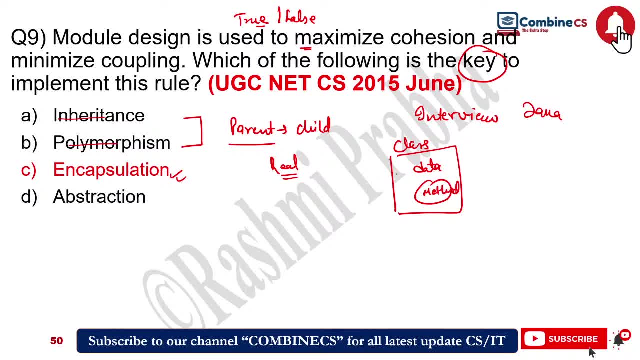 both are combined here. Okay, In one class you have data, that is, members and methods, So this is known as encapsulation. So what will you do in cohesion coupling? In cohesion coupling, when you do designing, there are different modules. 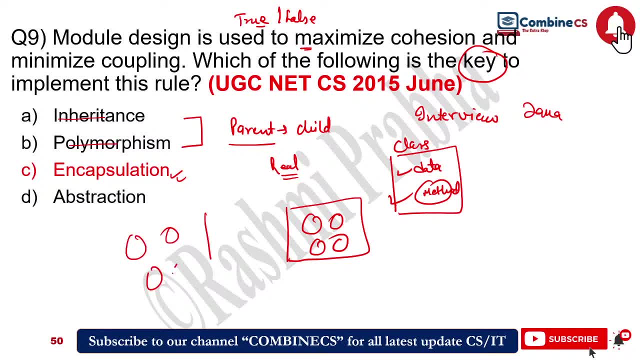 Either they are in one component, otherwise they will be like this: It means you are combining the features. That's why it is encapsulation. Abstraction will not happen because of this. Even if abstraction happens, you have to keep two things in mind here. 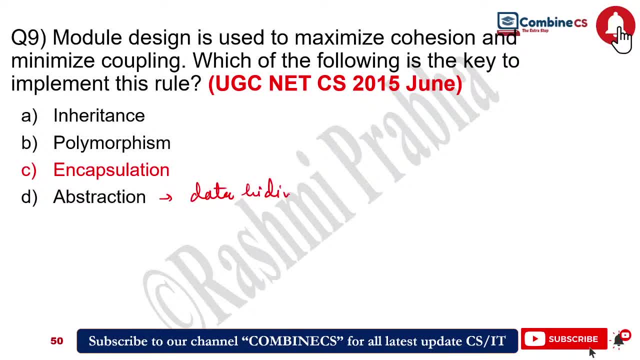 One concept is data hiding in abstraction, And the second concept will be: abstraction means whatever irrelevant information you have, that is, whatever the customer does not need. you will not reveal that to the customer. Okay, The simple thing is go to Amazon and place an order. 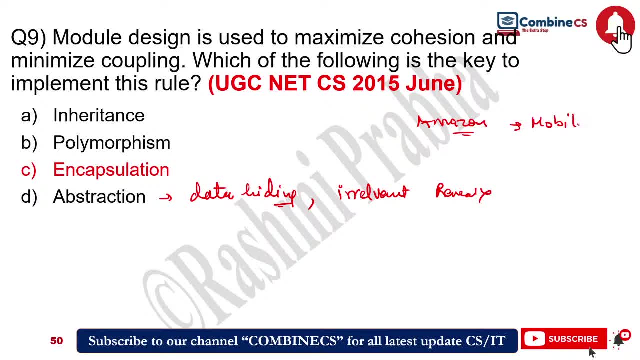 Suppose you have purchased a mobile from Amazon. Now, what are you doing in Amazon? First, you are selecting the mobile category. wise, Okay, You are putting many filters in the category, Filters in the sense that you will put your range. 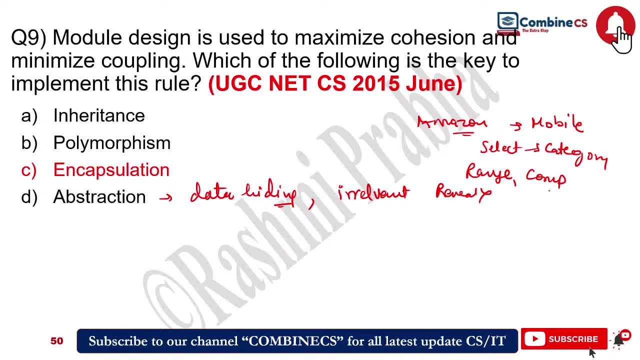 You will put the name of the company there. After that you check there. what are its reviews, What is its pricing, What is its color? These are the filters. How are these filters working? Sometimes you think, how is Amazon working so fast? 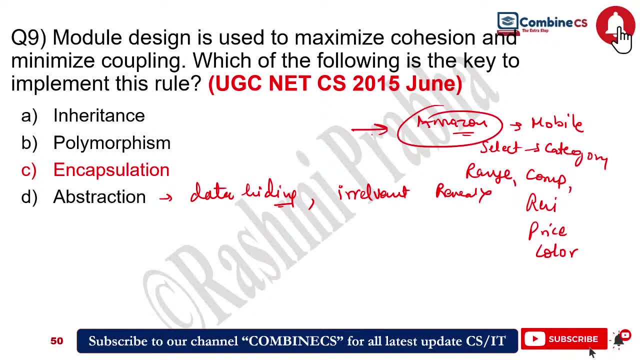 So somewhere the backend of Amazon, somewhere the backend of Amazon. they have implemented the backend so strongly that your search is very fast, Correct. So the meaning of selection is that, because I am a layman, what do I know? 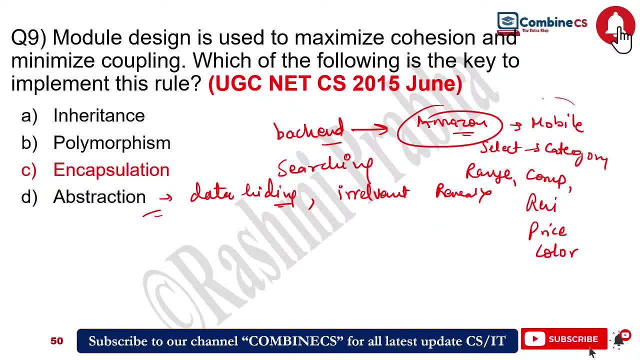 how is he doing the algorithm? My simple motive was that I want to buy a mobile for Rs 20,000.. So I went to Amazon website, I selected from there category wise and I paid for the mobile. So 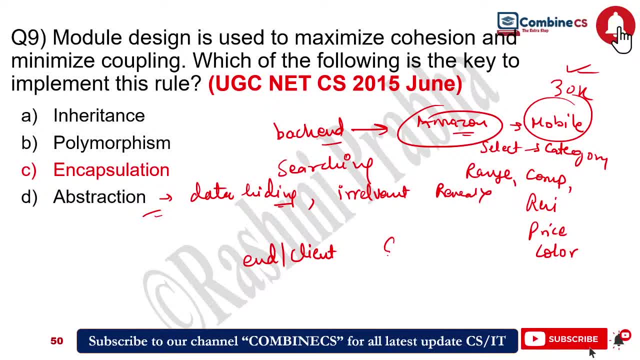 this is how your end user, whatever internal work you are doing, it should not have any meaning, Right? So in this question they have simply told that, module design In module design, your cohesion should be maximized and coupling should be minimized. 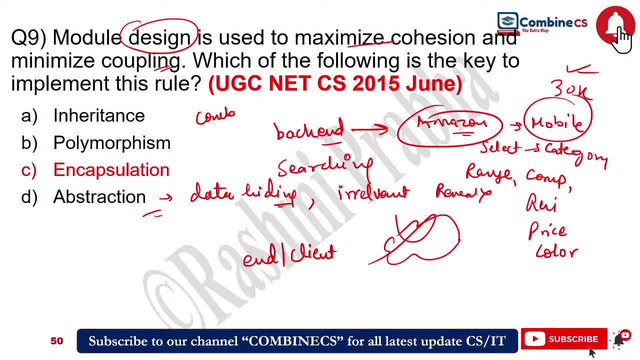 It means that you have to combine many units somewhere. So that's why its answer will be encapsulation. So this is how you have to. I guess there is some technical issue. This is also correct Now. 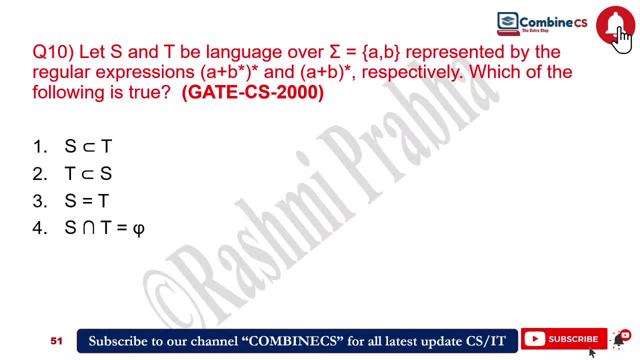 now give your. So what will be the answer of this question? I was trying to tell you why I put on this question is because in November 2020, if you have given the exam, then this same question came. You can check this. 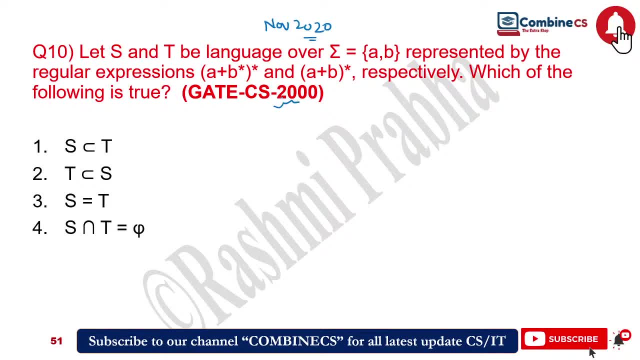 Somebody asked me: my learner asks how many previous year questions I have to ask. Now you suppose this is a question of 2000,. now you are having 2021. So any educator can't tell you how many previous year questions you have to ask. 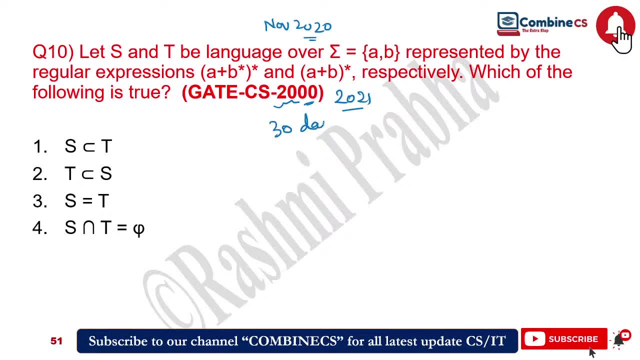 The thing is, if you have 30 days, If you have 30 days, If you have 30 days In 30 days, I am always telling you to ask at least 15 previous year questions And ask those previous year questions in such a way that you can ask every question related to that. 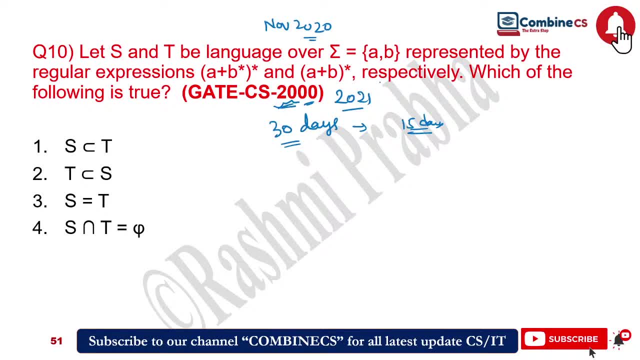 So this question was asked in grade 2020.. This question has been asked frequently in every exam. I am sure that this question has been asked in between, after grade 2020.. But this same question came in November 2020.. It is a simple thing. 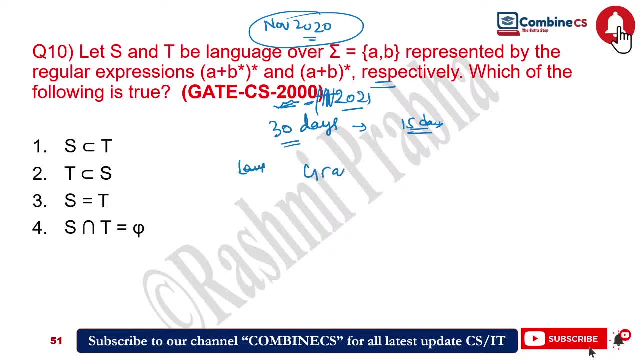 In this. you should know how to identify the grammar. Suppose this is written: A star plus B, So this is a property. It is a simple property that if you put a clean closure on any character, It means a simple string will become an epsilon, which is a null string. 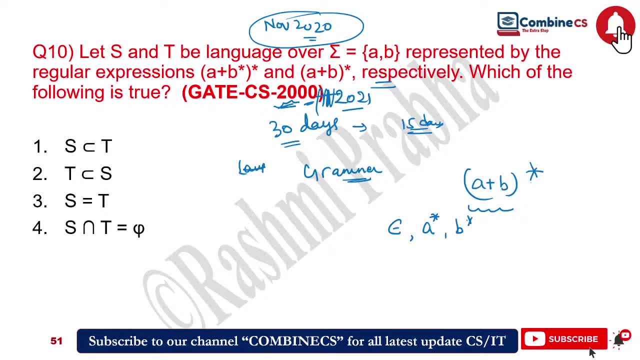 After this, you can make any combination of this A and B. You can make anything. You can make epsilon A, B, A A, B First. you can make B A A. You can make anything in any way. 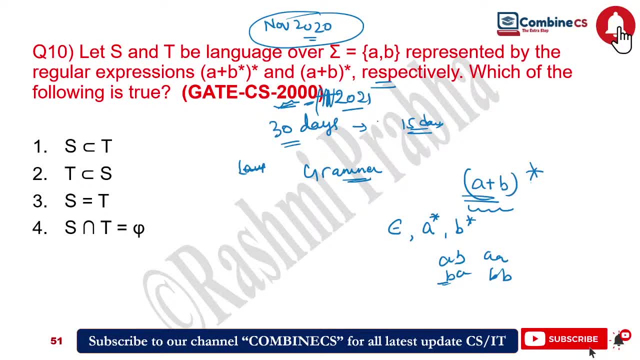 After that, when you study properties- So in properties this property is just equivalent to B star- You write like this: that both are same. Here a simple option will come. Option 3 is the proof statement. Here there is no mention of proper subset. 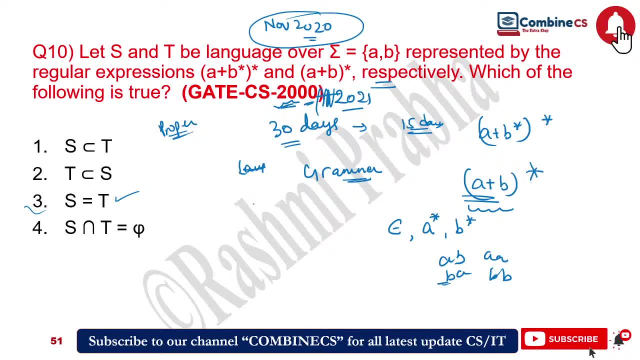 So there is no mention of proper subset. So here there are many statements. Let me write here: If this statement is given, Yes, if this statement is given, So you can write it like this: All the values will be same. You can write it like this: 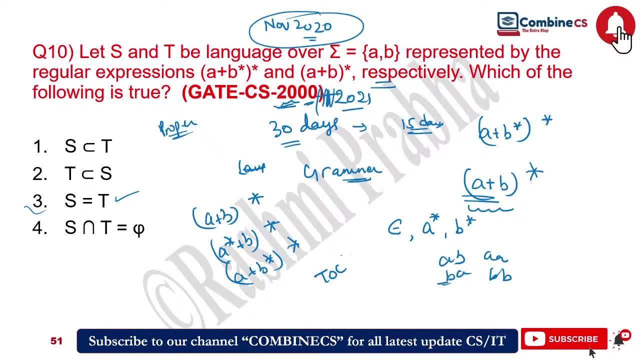 These are the properties, And those properties we have already covered in TOC videos Hardly. it is 14 to 15 videos on our channel And in that I have covered all the important topics, Which is very important from the perspective of your NET exam. 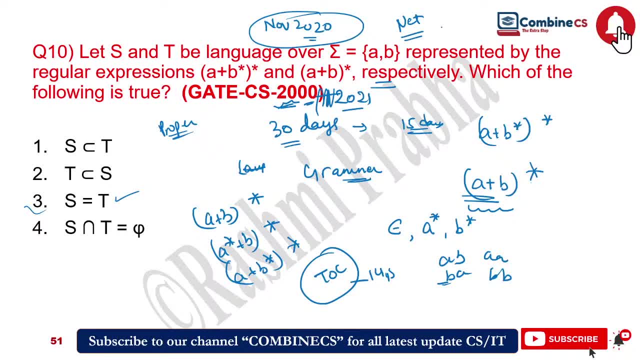 I am not talking about GATE, I am talking about NET, Because in NET you get predefined question That you should know how to identify language, You should know how to identify grammar, You should know PDA, You should know some decide EDT property. 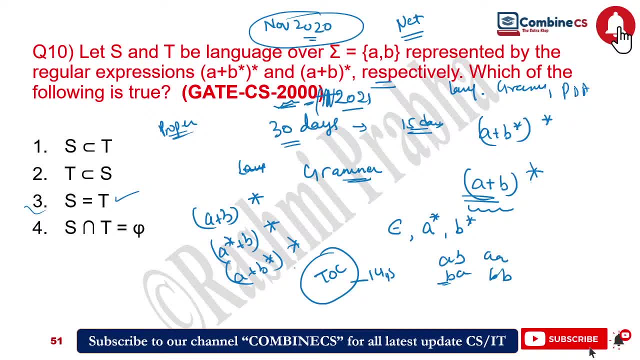 Closure property. Everything should be learn Correct. And after that you can write it like this: All these statements are same. This is a property. This is a property of clean closure- Correct. Write it like this: Everything is same. How much time will it take you in this question? 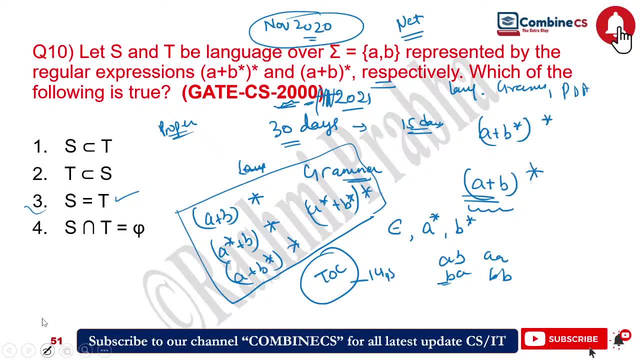 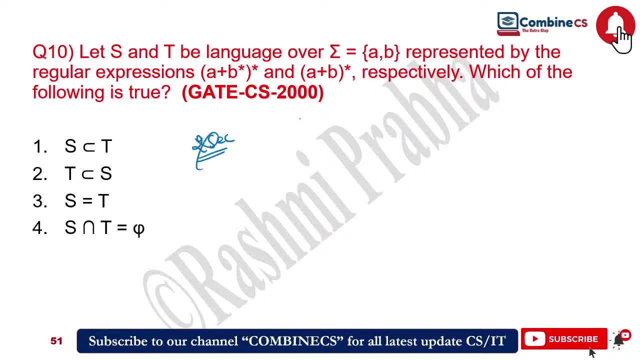 All the learners cry that time management is a big problem. If you solve this question, Let me tell you It should not take more than 2 seconds, But obviously Never solve the question in 2 seconds. Take time of at least 10 seconds. 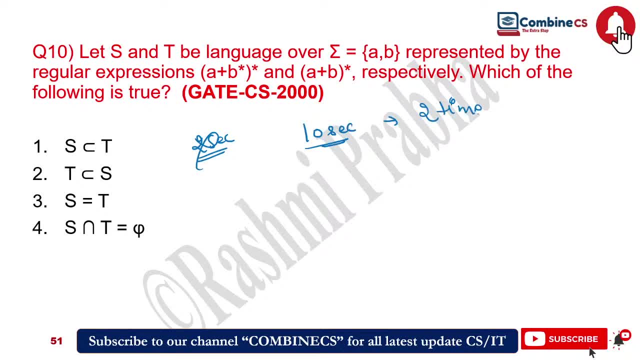 If the question is so easy, Which you have already studied, Still do it twice And before you press it, Also pay attention to which option you are selecting. There are many learners who knew that this option is correct. Still they put this option in the exam. 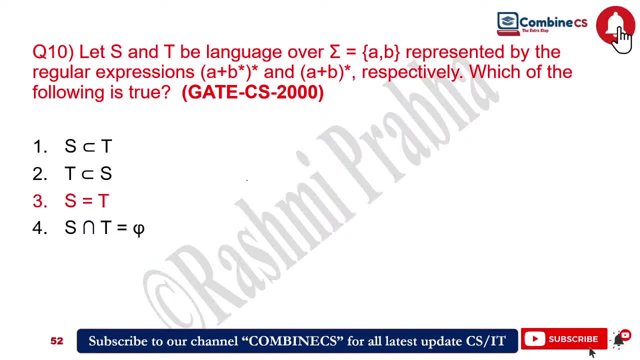 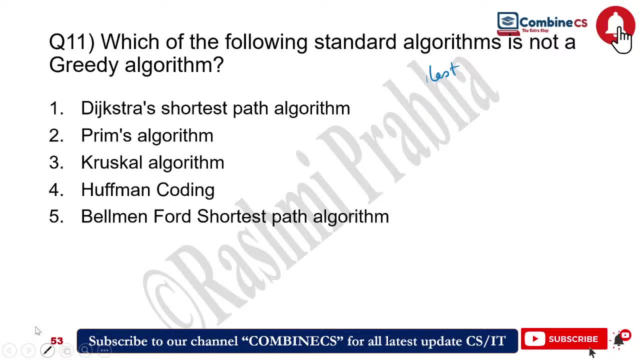 You should not make such a mistake. Okay, Now, This is the last question for this session. Basically, I am highlighting the important topic That how you have to learn. There is no any tough subject. Okay, It depends on how hard you have studied this subject. 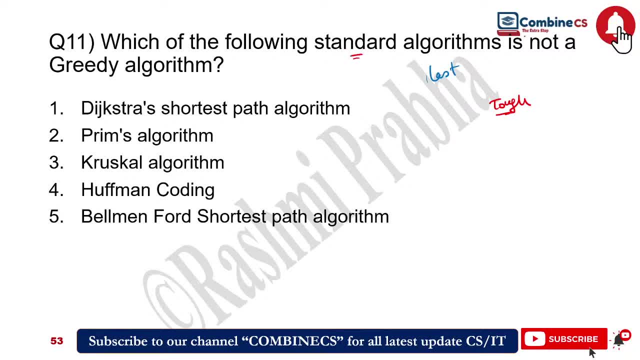 And how many questions you have solved. Which of the following standard algorithm is not a greedy algorithm? Read the question very carefully. Greedy algorithm, No. Now, there is no need of any concept in this question. If you know, This is hard coded question. 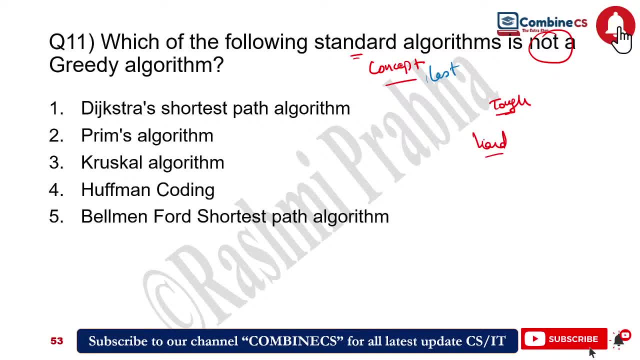 If you know, Then it will be correct. Otherwise, If you make a mistake, Then it will be wrong. Okay, So we have covered in this video: Hoffman, coding, Kruschikl, Tims, Always questions are asked And decast studies. 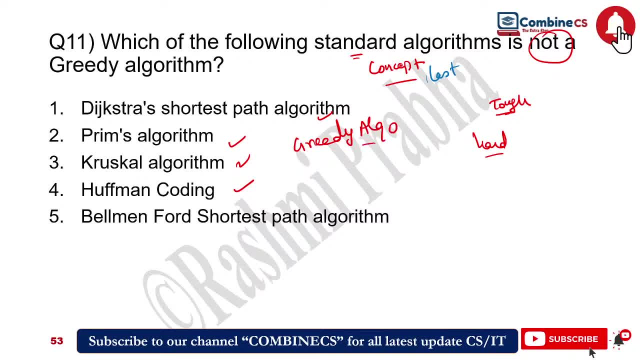 All are greedy algorithms. This is all a greedy algorithm. Just now I had started the session. That's why I have told Hoffman: coding is a greedy approach. Now How are you telling option 4.? Read the question Here. I have asked not. 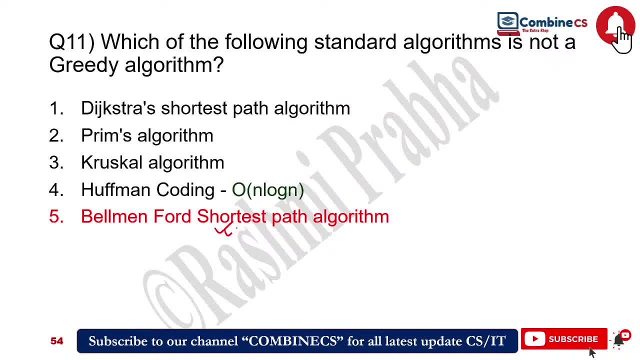 So option will be 5. Bellman-Ford-Sodden-Spark algorithm. Okay, This is not a greedy algorithm. You must maintain a chart, Write that chart, Stick it somewhere And see it daily once in the morning. 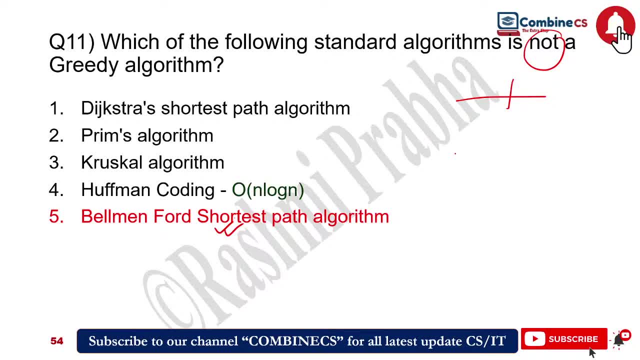 So this is how, In today's video, We have covered Hoffman coding. I have given you two assignment questions, So you can pause the video And provide me the answer to that question. Otherwise, You can join our whatsapp group Or you can join our telegram group. 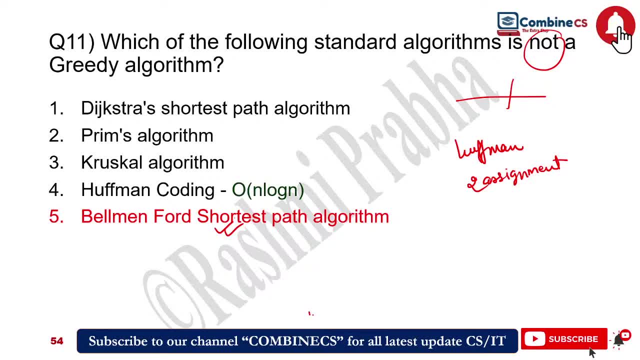 Where I will send you a screenshot of this question. You can solve it from there And give me the answer So in the video. If you think That I am doubtful in this topic, Then you are in the comment section of this video. 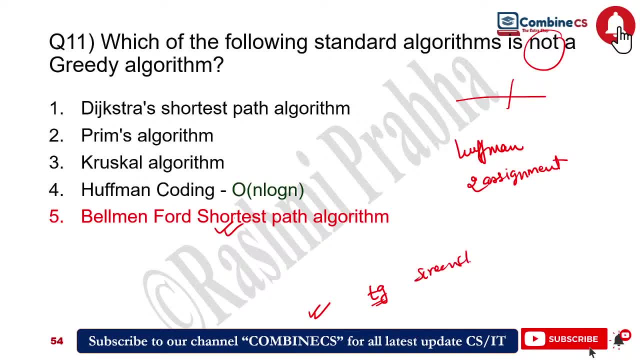 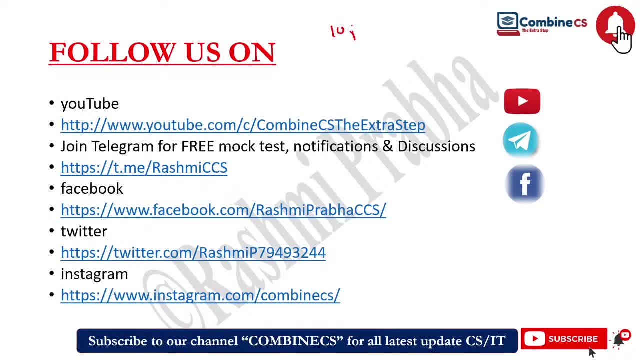 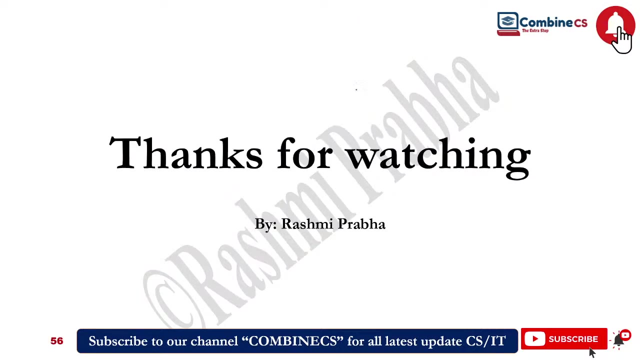 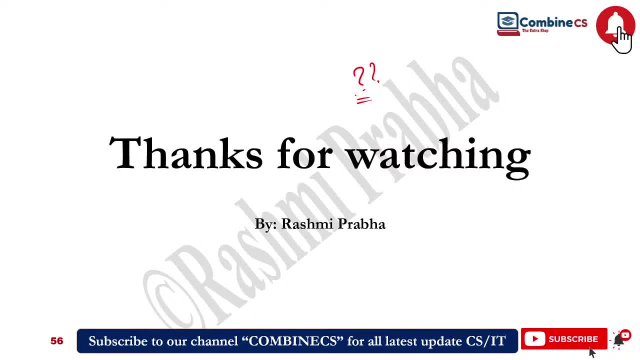